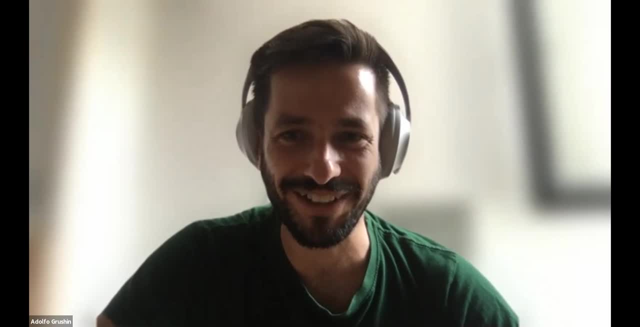 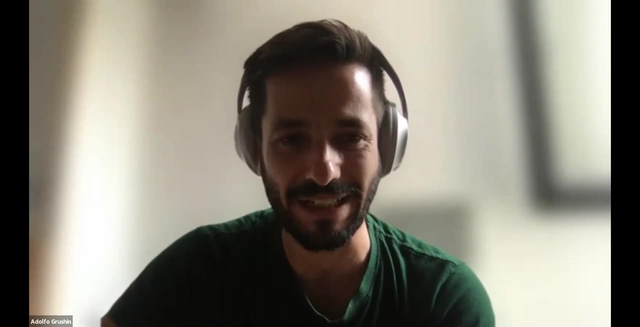 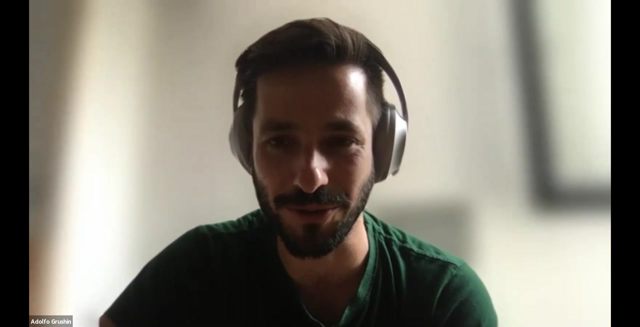 she's very well known for growing every material in town And in the world that does anything topological. And yeah, I mean, feel free to share your screen and the floor is yours and we're very excited to hear what you have to say. 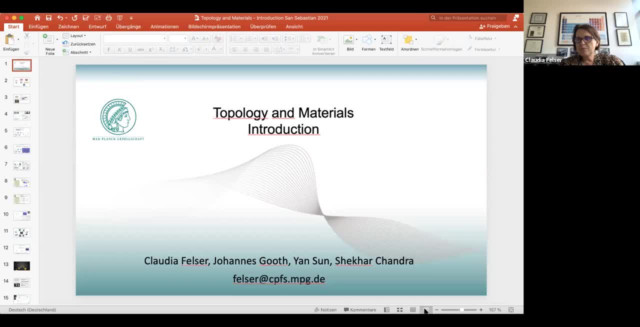 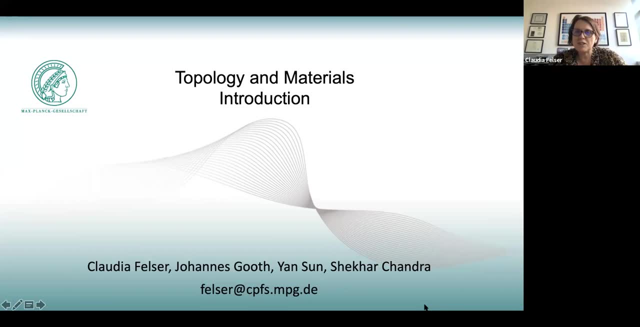 So I'm always the relaxing part of the conference- right, because this is mainly a series conference and So I'm always the relaxing part of the conference and I'm going to spread with a few experimental- is showing you what you can do with what you learned, what you can maybe also tell us what to grow. Okay, so I will give you a little bit an introduction and I focus on topology. 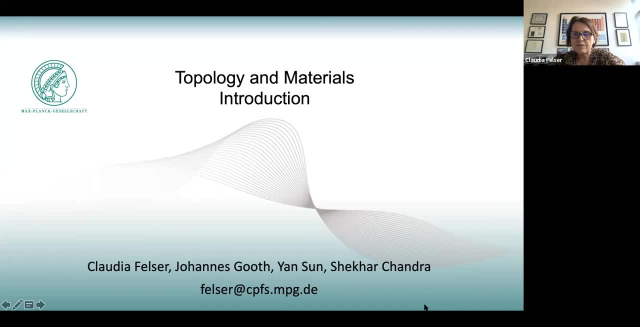 I make small bridges to ruffian and maybe just perfect. So, because this is already question, I'd offer you in chat with the question, right? Okay, so I focus on topology. Okay, So I focus on topology so everybody can lean back, relax and listen to what we are doing. 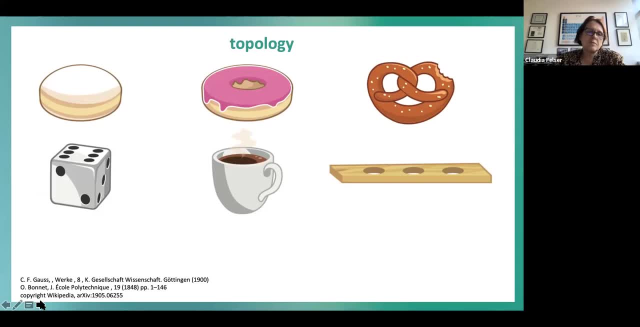 Now I hope it works Okay. so so you are familiar with the concept of topology, but I still put this slide in because I have seen mainly all the talks were about twisted graphene, but this is also seen, can be seen in the context of topology, and you know we all look. 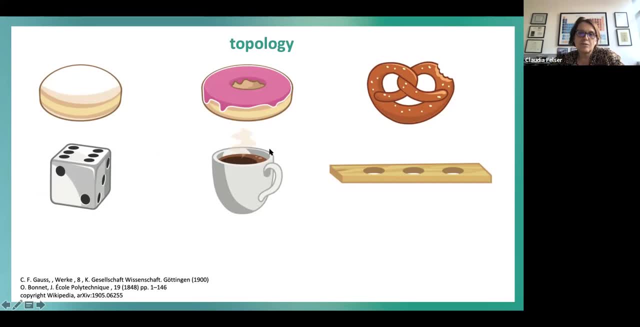 for for the topology of objects and I like to show you. Okay, So I like to show our picture of the topology of object. so, like this: for example, donut has the same topology as a coffee coffee pot, as you know, because both have a whole and the bread, so he has three holes and this is the same as this. 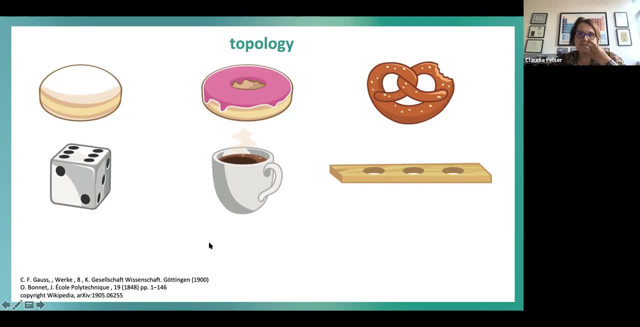 And this we can apply to not only this object in real space. we can also try this to the electronic structure and reciprocal space, And so, and this is all about topology And this topology And this topology. So I think this is, this is a very interesting story started. 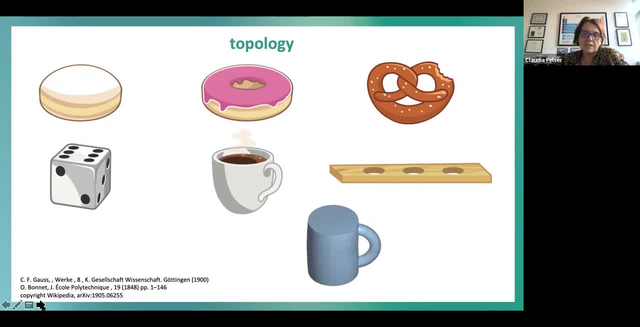 Now 15 years ago, more than 15 years ago, and I think it really has revolutionized solids And I think it's not so far. we only see the tip of the ice pack, even when we include the twisted graphene. So I think we maybe can come via twisted graphene also to molecules, organic molecules, and find even more topology and organic reaction or chemical reaction in general. 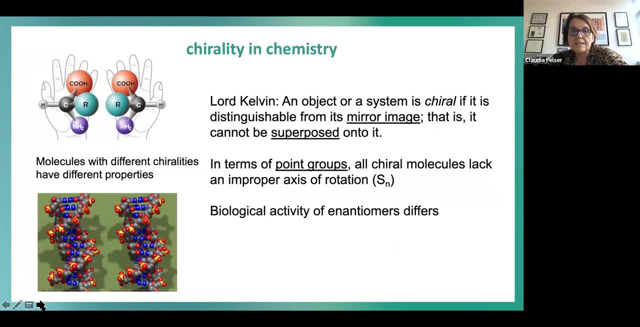 it might be interesting in a much broader way. so, and if you want to ask me what is most exciting thing in chemistry, so i'm also a solid chemist and more on the physics side, but the chemists are mainly excited about chirality of molecules, organic chemistry, because they show very 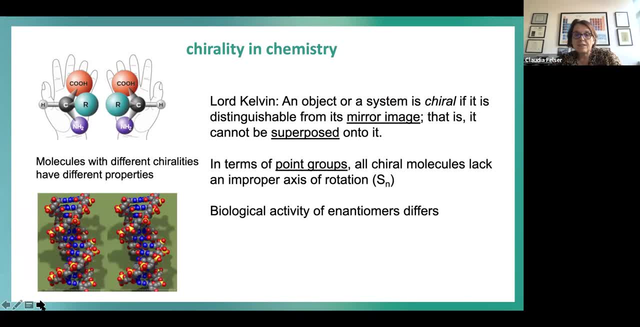 interesting properties and they are very distinguished only under a certain viewpoint. so because you can make these two molecules which have exactly, for example, the same atoms, and since the carbon is coordinated tetrahedrally, so the two molecules, you can make two different molecules if you have four different ligands here on these carbon atoms, which are like the hand, the right. 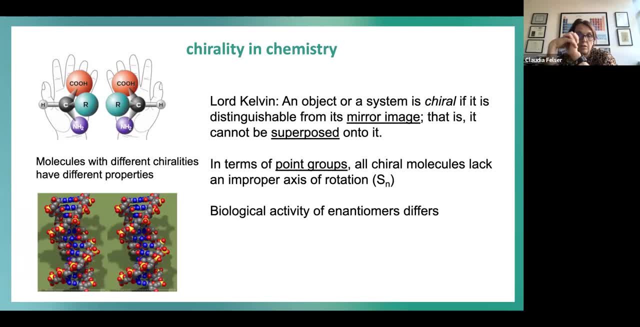 and the left hand and they cannot super post onto it. and so this is the basis for life, because all the molecules and life ends are given, and even the bigger macromolecules in life are chiral And the processes like motors in cells are chiral. 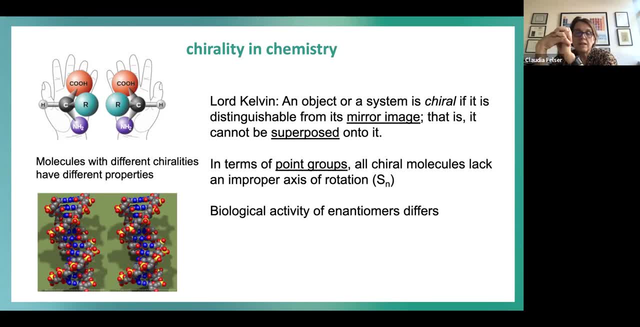 So chirality is extremely important in chemistry And this is a viewpoint of topology in chemistry You have seen the first figure more related to mathematics, And it still is a very open question how we fundamentally have broken symmetry in life, because we all exist only are made by left-handed DNA. 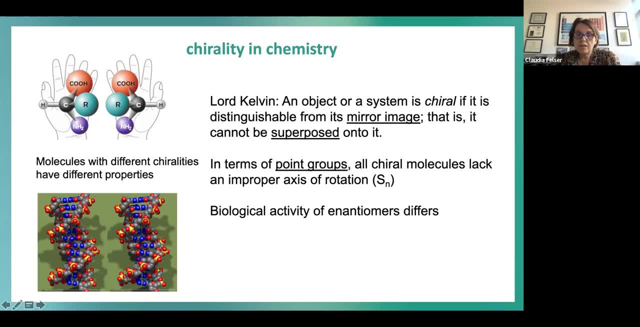 And we are eating only right-handed sugar. And it's not so clear how this fundamental, broken symmetry has appeared on Earth. And it's one of the biggest questions I still think we have to ask. And maybe there is a connection between the topology we are thinking here in physics also. 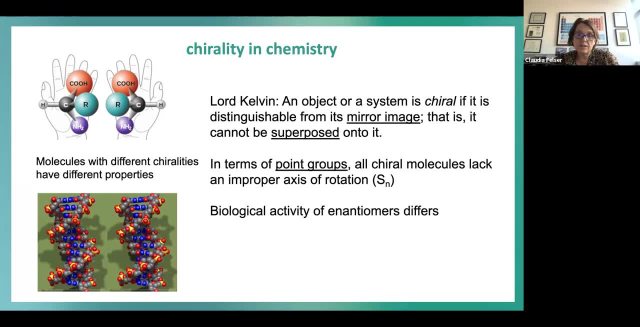 And one of the. here's the first one of a bigger chiral macromolecules. One of the molecules you learn about is the twisted graphene. Twisted graphene will always described as twisted graphene, But you can have two twisting angles And this gives you the two different enantiomers. 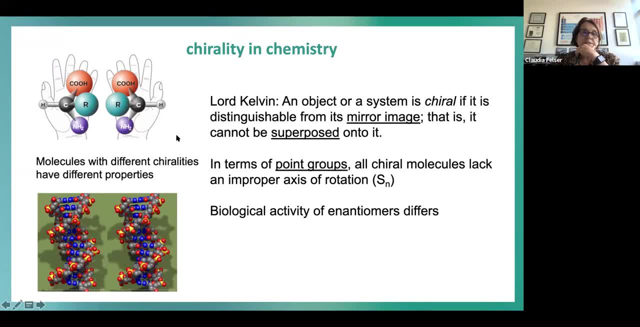 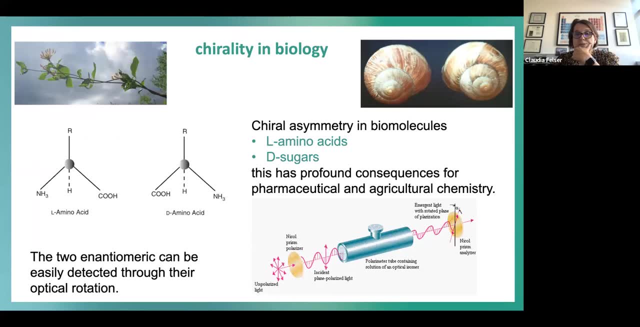 So, like in the right hand and the left hand molecule twisted graphene can have the right angle or the left angle in the sense also twisted. So this is really interesting And you can even have macroscopic object like this here which can be charged. 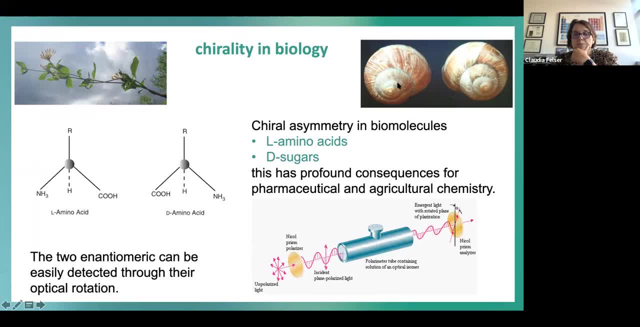 by the. And the only way to distinguish, for example, two different amino acids which have different chirality is by do it optically, because they, they, they, they, you know, change the rotation plane of linear polarized light in different direction. 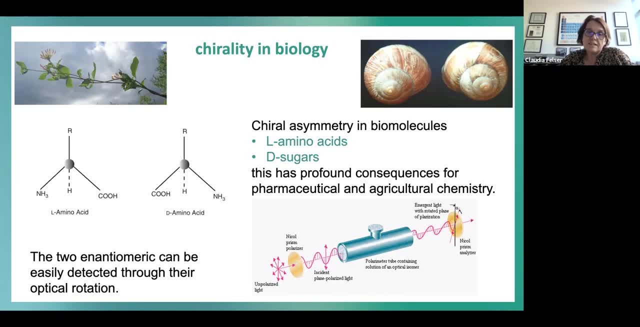 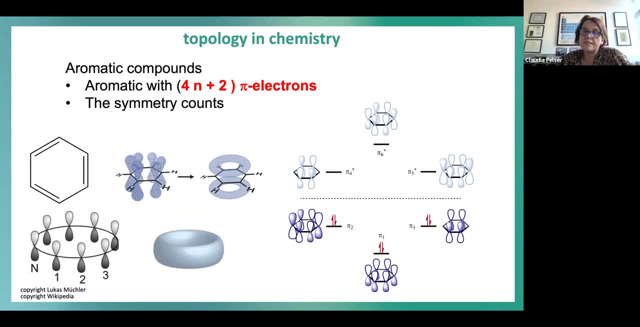 And this is why they got the names right and left handed And it's whether they change it in the right or left direction. So there are other ways of thinking about topology in chemistry, And this is a slide which Lucas Mischler made. 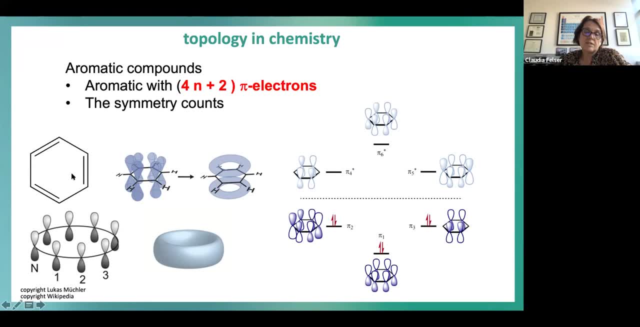 And we discussed this. So there is also an organic molecules, And here We start with the first building block. This is also the centric building block of graphene. This is benzene, So the, which has six carbon atoms here and one single bond. 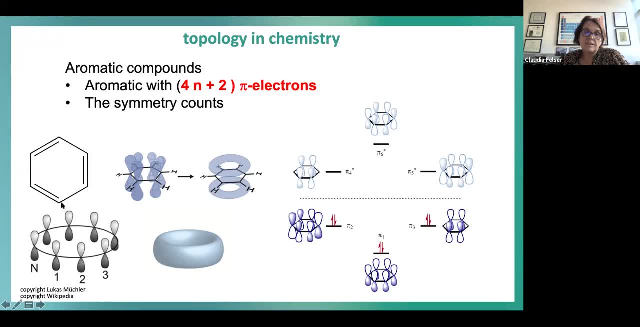 and one double bond. But this picture is the KQD formula is not the right picture, because if you would draw it in a different way, here with this, only these orbitals which building the double bonds here, the so-called p orbitals. So we have here again the carbons and the hydrogenates. 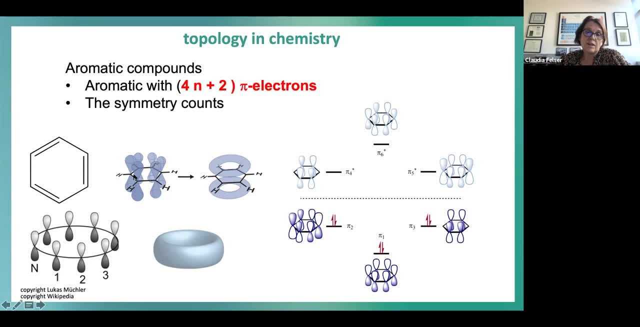 Which you don't see in this drawing. So then you have: the bonding are all the same length, So there's no distinction between double and single bond, like you would think here. So and the electrons are delocalized in benzene, So this we call aromatic. 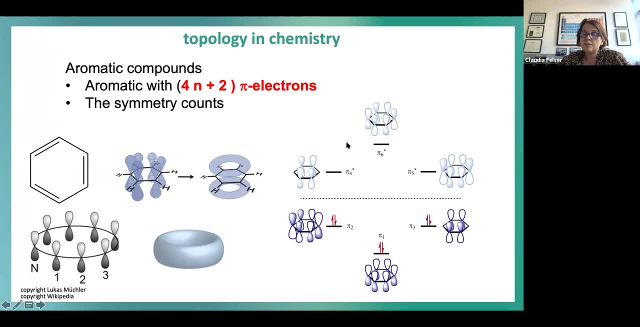 And there are simple electronic counting rules which are depending on the molecular orbital diagram of this molecule. So this are all molecules Which have single bond, double bond, single bond, double bond kind of arrangement. So you always have aromaticity if you have 4n plus 2p electrons. 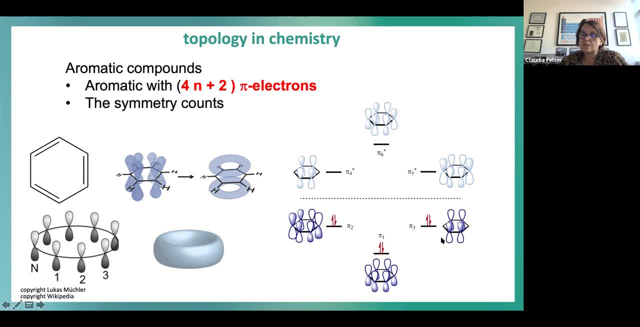 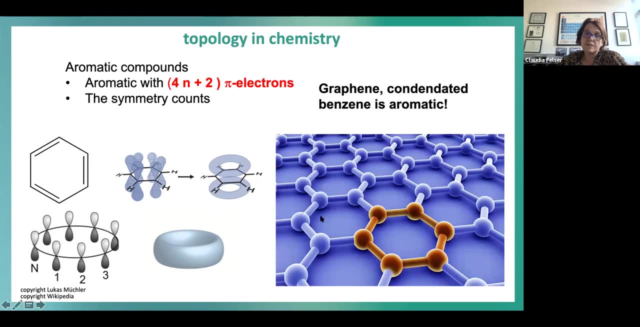 Because then you have filled this degenerated state here, And this is interesting because this can. this is a building block of graphene, And graphene we can understood also as a totally delocalized p electron system, So it's like Many benzene rings, condensates. 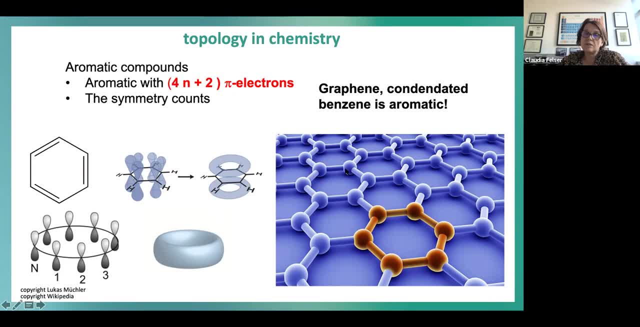 So we have not telling. if you have two inorganic chemistry and we have an infinite number. we have graphene. So graphene is an aromatic molecule. It fulfills the 4n plus 2p electron rule. So what chemists like to do they like. 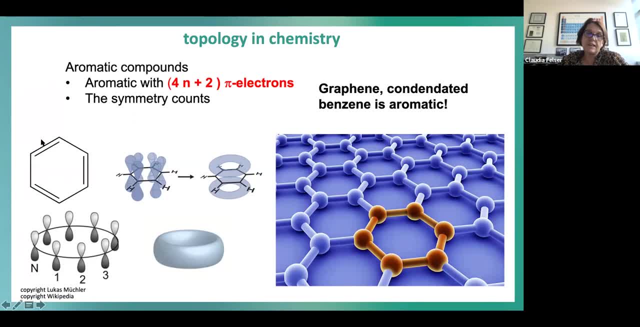 and if you have, for example, rings- which I have- eight carbon atoms and four double bond, they're not aromatic. Even you could think on the first view they are aromatic. They are so-called anti-aromatic. Here the electrons are really localized in the double bonds. 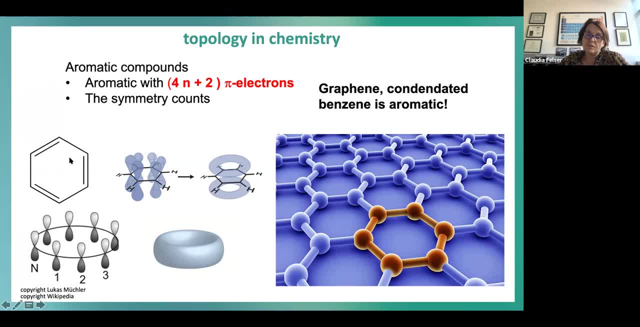 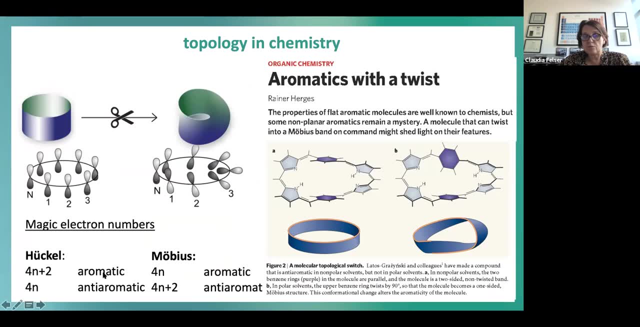 And so they are not delocalized over the whole ring. So these are the so-called trickle rules: that you have 4n plus 2 electrons to be an aromatic molecule, And if you have only 4n then it's anti-aromatic. 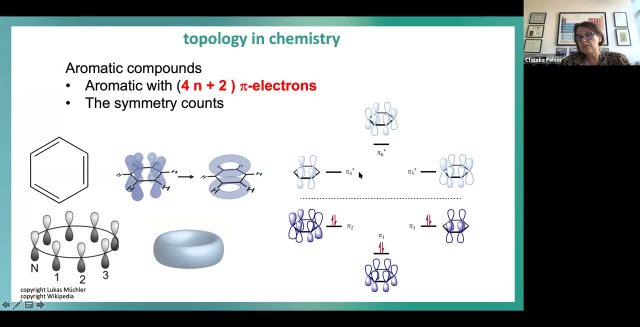 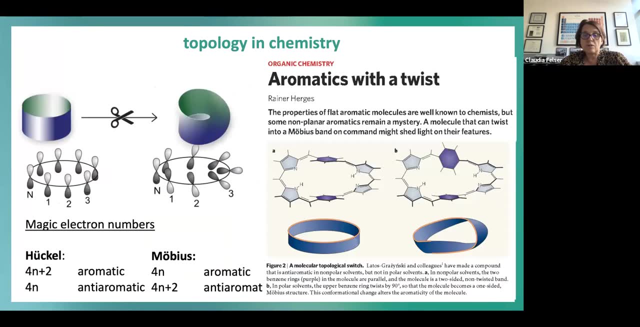 And this is related to the electron diagram. You can imagine if you fill this half. it's not this best the stabilization to have this delocalized, Okay, but what happens? and this brings us to topology and you will see to the difference between doughnuts. 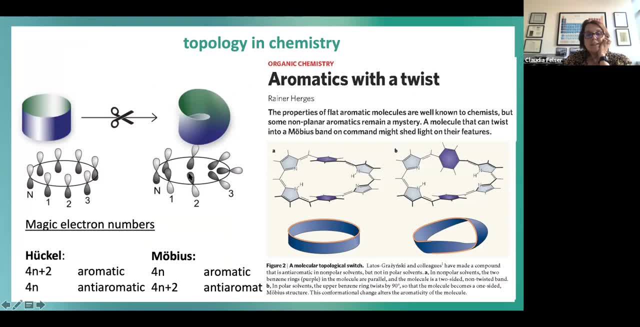 and Möbius stripe, which we will discuss also in solids, is like if you would make a twist in these molecules, and this is possible. organic chemists can make this twisted molecules. this rules for whether something is aromatic or anti-aromatic- unworth. 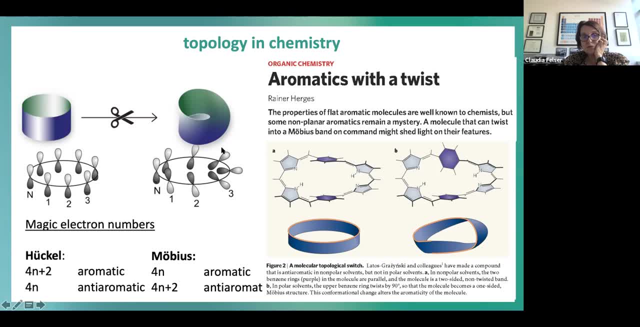 And this is related. So if you draw the orbit, if you draw the orbit, so you have also to draw the twist, and this is related to some resonant orbitals. If you do a tight, binding model calculation, you can explain it. 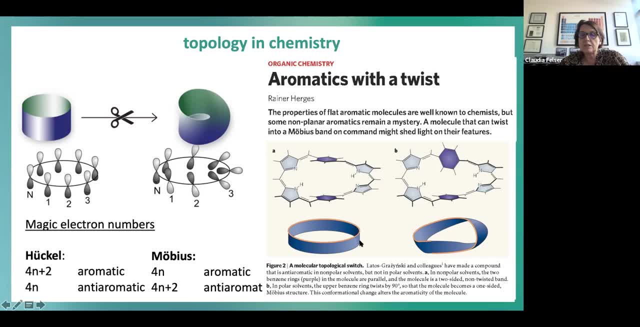 So, and this is possible, So we can make molecules which are more like a doughnut and which are more like a Möbius stripe. And you see, in the optical properties even the atoms are exactly the same in both molecules, that they are different. 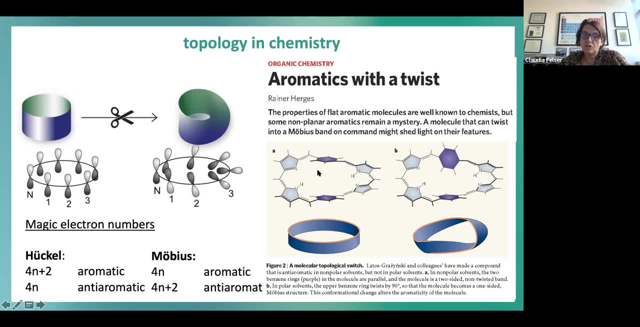 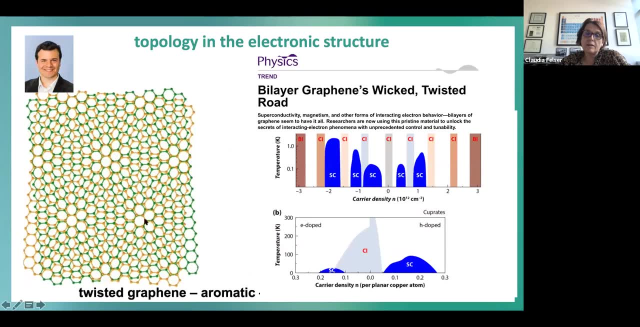 So from their optical properties, because of their change in anti-aromaticity, And in this sense we, as from the chemical view, we could also understand this, so that twisted graphene, now from graphene, is aromatic. It has this very nice flat delocalized p-electron sheet. 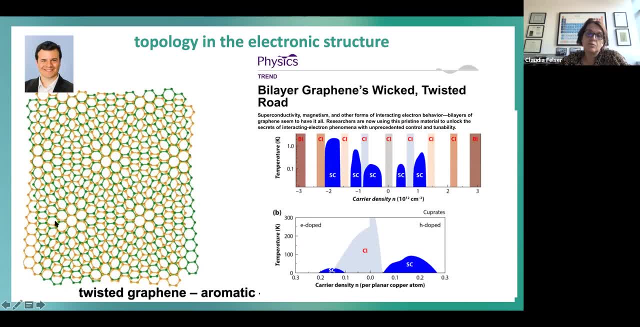 And then, if you twist it so you get interactions between the two layers And you would explain it by all the nice models with thread bands Et cetera. But you could also interpretate it that you now have areas of anti-aromaticity. 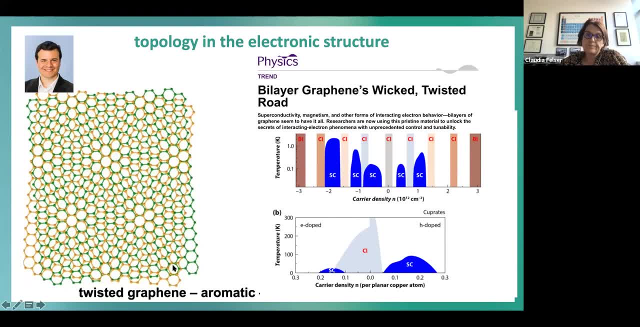 because you now have not really delocalized electron contribution And this might explain that we have this correlated insulators in graphene And the question is here: can we use the same for describing organic and inorganic compounds? And, as we learned today, there's also 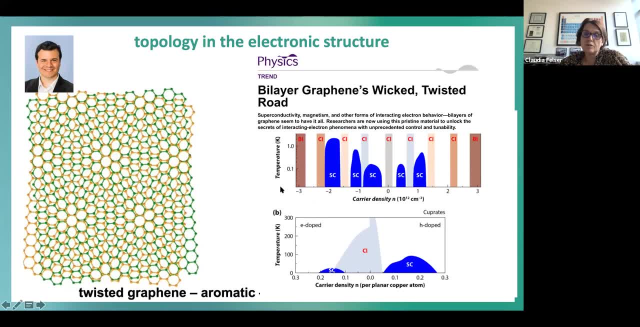 that you see many, many more interesting properties like superconductivity, et cetera, in twisted graphene. But you see already there is a way to chemistry which is not yet gone, So maybe we can even go from the solid via twisted graphene. 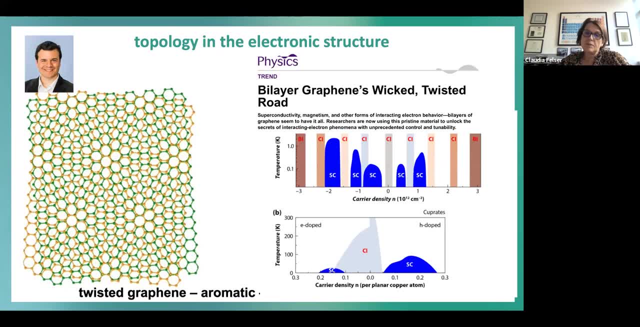 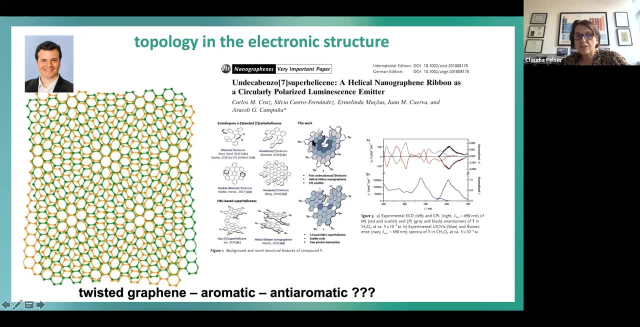 But I will focus on the solid, since this is my main speciality. OK, Here's another example which I still want to show. It's like that you can also make larger molecules Which look like a smaller sheet of graphene than the sheets we use nowadays. 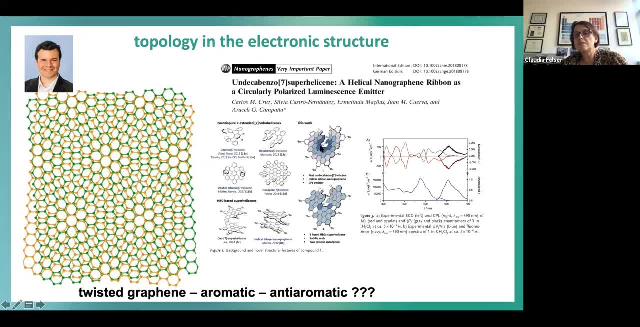 And you can give them, even by chemical synthesis a twist. And also here you can twist it in two directions And the luminous sense of light. light is different for the two twisted candidates, which already shows that there's a nice light-matter. 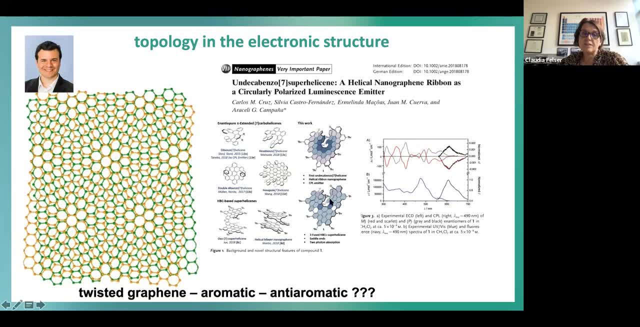 interaction And there is really the twist with the same electrons also here- Makes a nice difference And it's also again a bridge- nice- from solid-state physics via twisted graphene maybe, to chemistry, where we have much more to do. 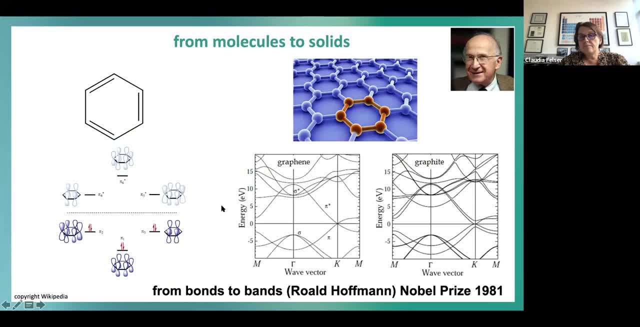 OK. So the important thing is also- and this is your speciality- to see the band structure, So like going from molecules to bonds. So more or less The band structure of graphene can be understood in a similar way, by making nothing else. 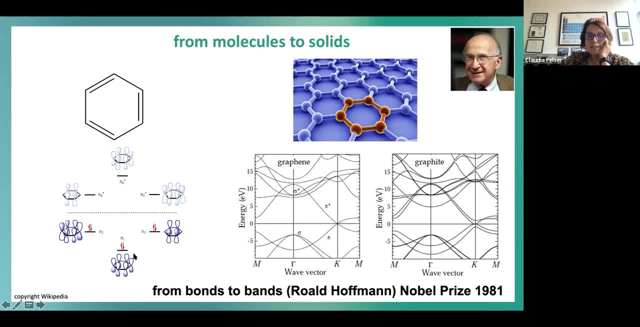 and condensating many benzene rings And you see, the bands are still related to this. We have the sigma-sigma bonding between the two carbons, But we have also the P-bonding here And these are the important bands here around. 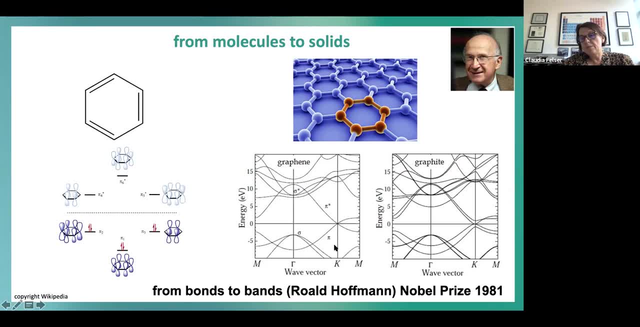 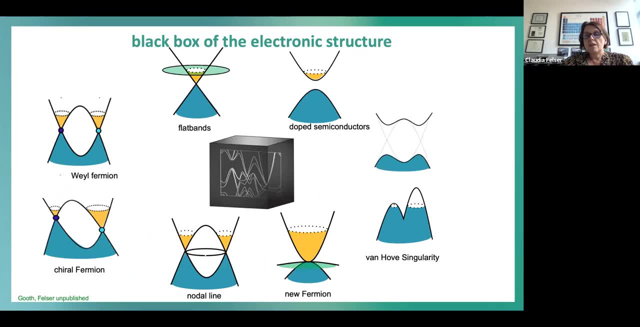 which leads to the gamma, to the K-point And the diracone in graphene. So what nowadays, I think, also is a new view on topology and especially also for us. So before we, the people who do also computational material science, they 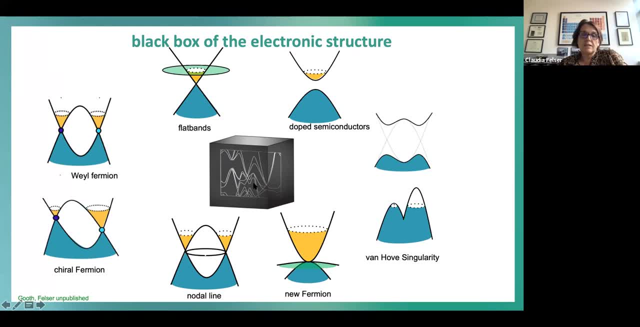 have simply calculated the band structure, And then you calculate some observables like the magnetic moment or the conductivity, how many, how high is the density of states, and so on. So, but we use more or less the whole band structure. 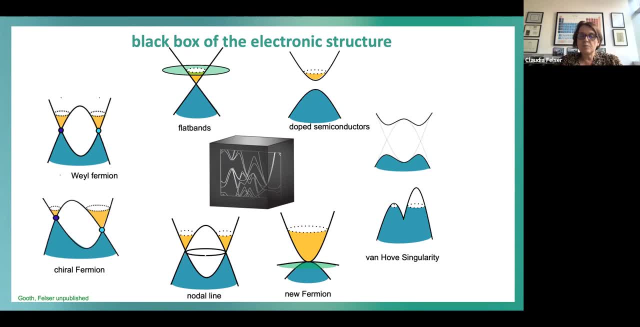 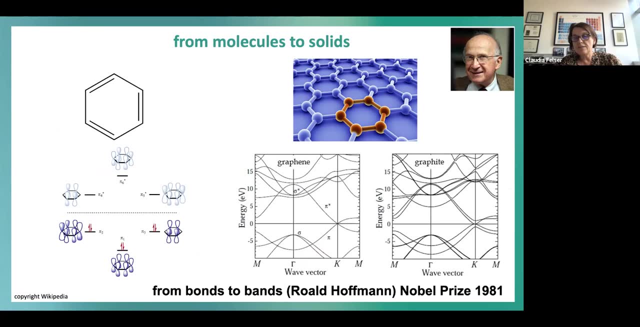 as a black box, But this was already, I have to say, a little bit different If you go to books and papers from Roald Hofmann, and this is what Leslie Lucas and me I love, and I strongly recommend this also to the physicists. 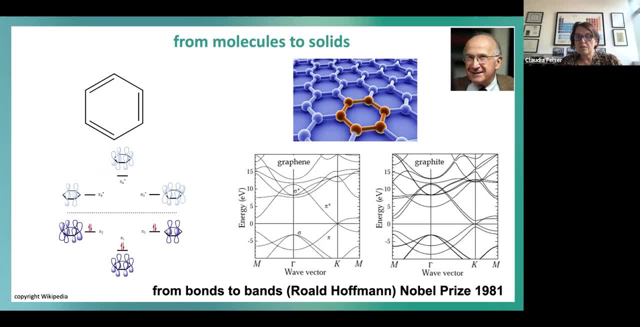 So he wrote very nice papers about organic chemistry and got the Nobel Prize for organic chemistry. But he also have helped us to understand inorganics, solids, from a very different view, by simply symmetry aspects, And this is more or less the basics for what we can understand. 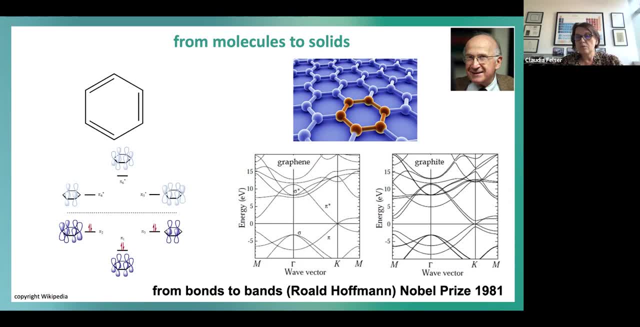 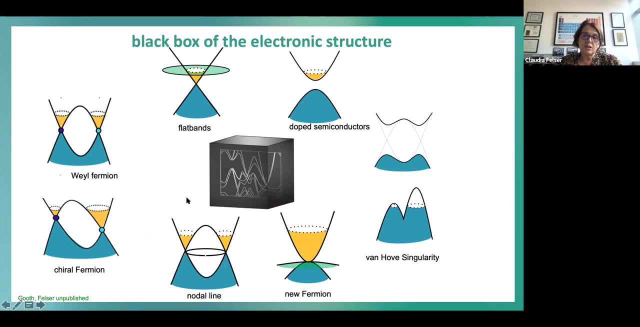 and get out of, And it's strongly related also to the concepts of topology nowadays. Okay, So already he looked for features in the band structure which can explain certain properties, And this is more or less what we are nowadays are doing. 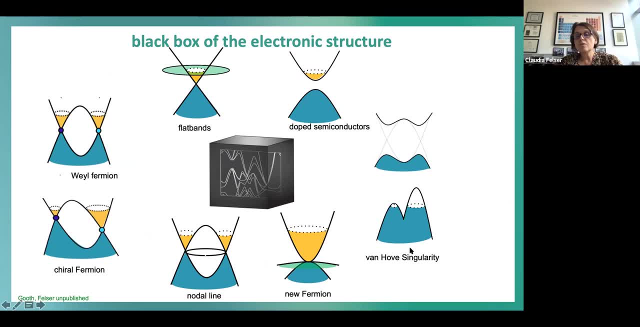 So like we like to see features, So in the past we also looked for van Hofer singularities. This was my PhD student time when we looked for van Hofer singularity to find new superconductors And nowadays the zoo of features which we are looking. 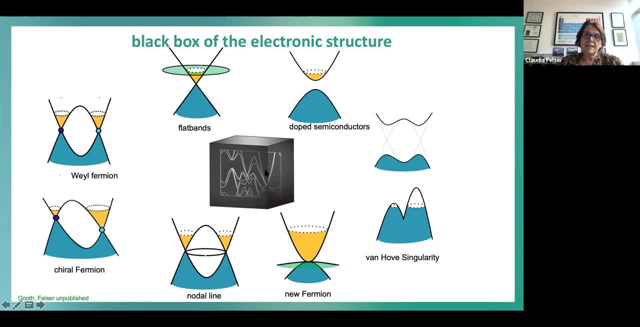 So we shine light in the sense into the black box of the electronic structure and look for flat bands, like in graphene, to find new interesting material. So it's a totally new way to see materials And this opened us to a pathway really to do super exciting physics on many of these materials. 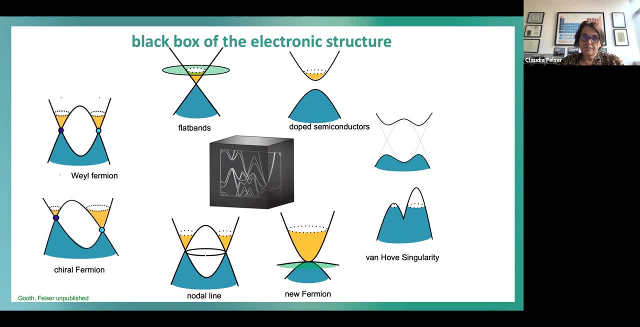 And still I think we are still on the top of the iceberg. So I want to a little bit shine light on different of these properties from the view One of the experimental, from the experimental viewpoint and, in the topology, experimental viewpoint, And I want to explain you a little bit. 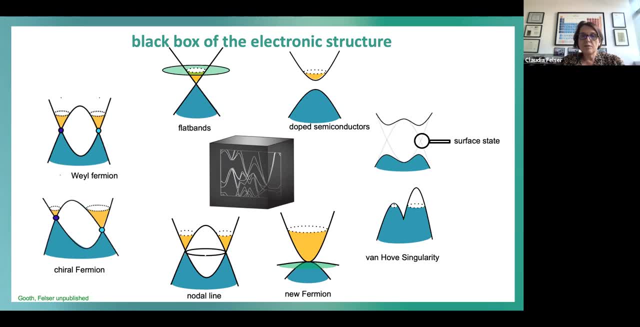 what we are doing in the world of experiment to inspire us as a theoretician. maybe few experimentalists are also here to come up even with more ideas. I already know I get many ideas from Maya and Adolfo, And recently I received a very nice paper from Jen. 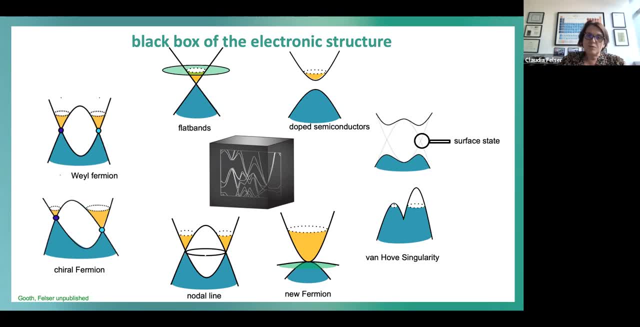 which I'm discussing now with the optics people. So this is the best way to do science and it's super efficient and it's a lot of fun And I think never in the history of quantum metaphysics it has worked so nicely that theory can drive the experiment. 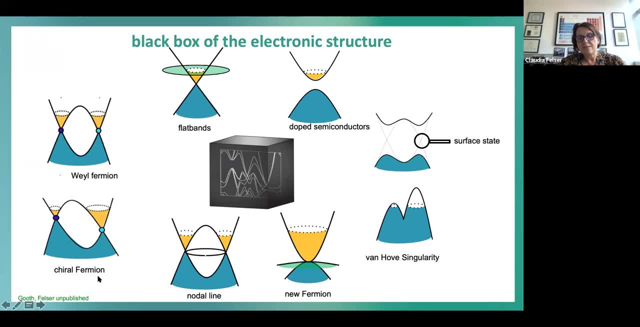 But since we now understand much more of the features in the electronic structure and still we don't. you see, if you see the spaghetti here, you see you recognize a few of those features, but there are many maybe unrecognized features or even hidden features. This is electronic structure. 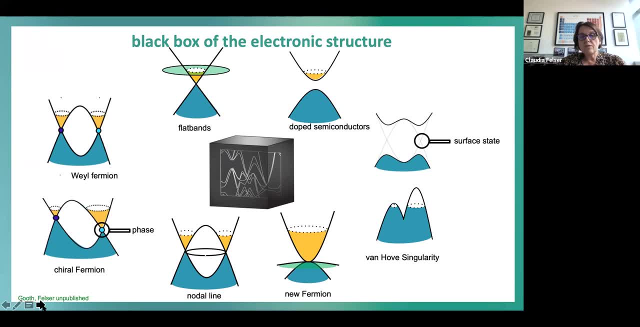 So, but what I think is also super interesting, we are now looking for surface states and for the phase. So this is when you- and this is my then also recommendation for the future. So we looking much more now on surface state, but looking also on the phase of wave function. 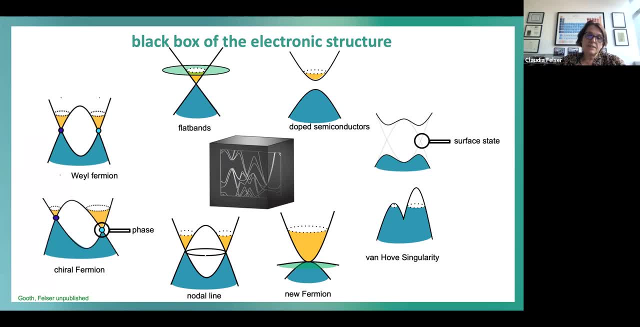 is not fully seeing the aspects, whether we can use a certain phase, And this is especially interesting in the viewpoint and as a viewpoint of chirality, because chirality is the electronic structure. the MO diagram of both molecules, both handed molecules, is exactly the same. 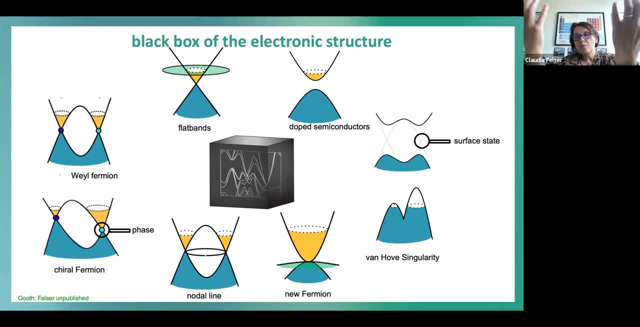 And this is also the problem, because this is the reason- the energy of both molecules is exactly the same, So it's not easy to separate them, And there's a big market, pharmaceutical industry. since we are all chiral, So also most of the medications are chiral. 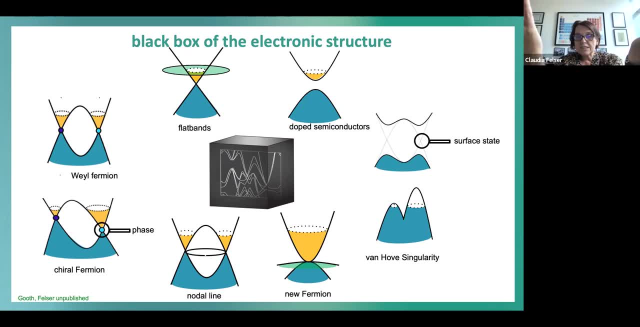 So it's very difficult to separate them. So, but the interesting thing is the surface state, which you will learn tomorrow, and the phase of the wave function are different, And maybe these are ways to take advantage and distinguish this: chiral molecules and chiral crystals. 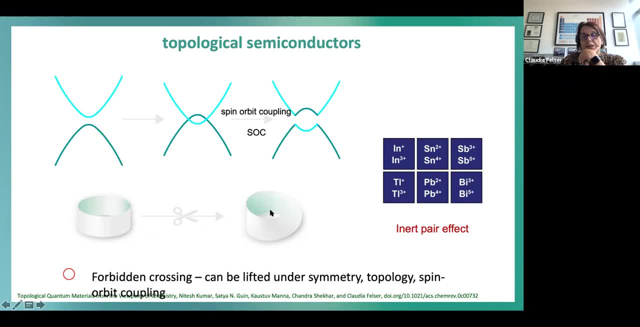 Anyway. so we mentioned already doughnuts and Möbius stripe and the basic concept of topological insulators, And I'm sure you are familiar with this, but I like to bring everything together to bring it in a more complete story from my viewpoint is like so that: 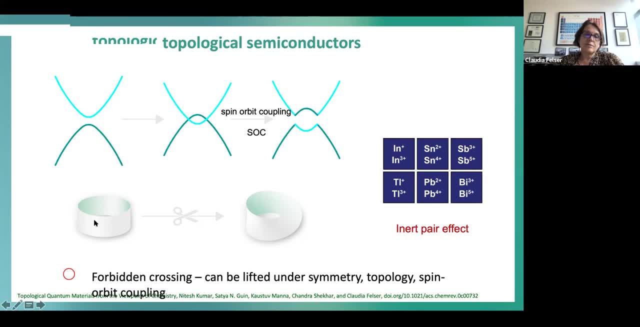 so we see this in the electronic structure, as I already mentioned. So in a normal semiconductor we have valence band and conduction band, which was the occupied MOs in benzene and the unoccupied molecule orbitals in benzene. But now, since we have solids, we have bands. 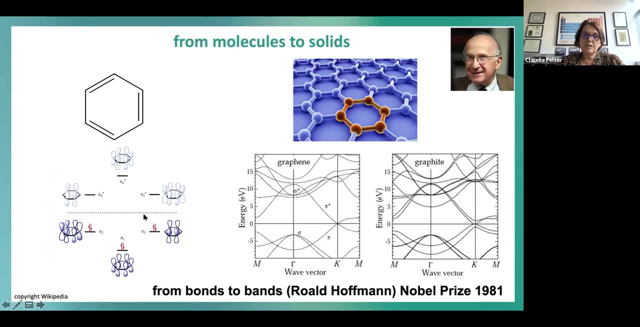 I forgot to say this, but I showed this already here. So here we have molecule orbitals, the occupied one, the unoccupied one for benzene. Here we have the same situation, more or less. Here we have the same situation, more or less. 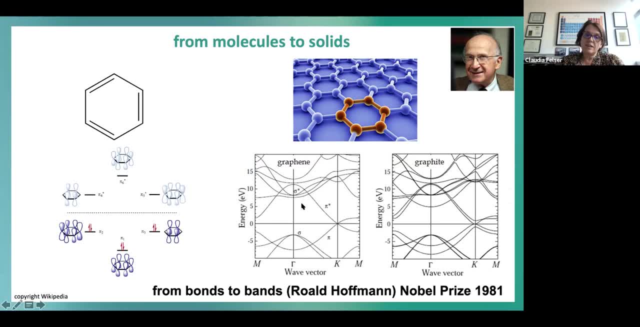 Here we have the occupied bands and the unoccupied band for a layer of graphene. They at the gamma point. they are identically with the MO diagram, But since we have translation symmetry, our bands get an additional phase. So we have therefore this very nice band structure. 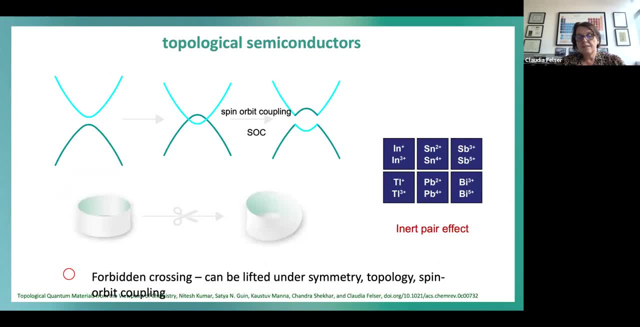 So this is also very nicely described also how to do this and even draw it by hand- the graphene band structure in this article. So this is also very nicely described also how to do this And even draw it by hand- the graphene band structure in this article. 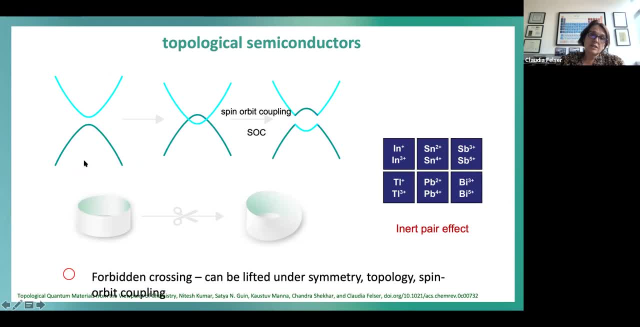 Okay, So, so we have this conduction and the verdant band now, since we have bands and solids and this, this, this the band gap. the gap between the occupied and unoccupied states depends on the bonding strength. So, if we have hydrogen, 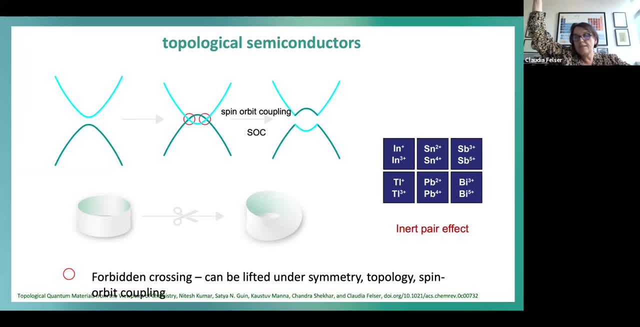 so this band gap is giant. So we have hydrogen, this gas tiny band gap, for example, compared to a cadmium celerite and then to a negative. We then we again change it, So again also. which is the, was the yellow color of the postcards in germany. so, uh, and you can, but also 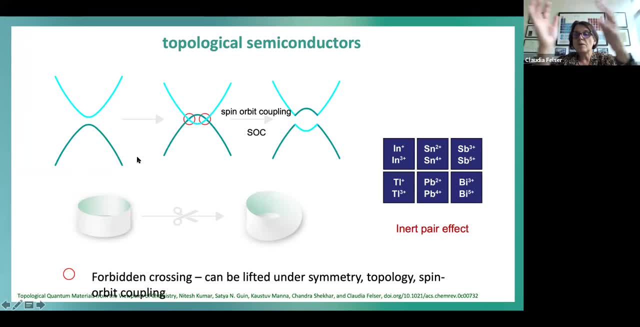 have the situation that the bonding strength, even in this binary systems are smaller, and then what can happen? that the conduction band and surveillance band overlap. so we have this so-called forbidden crossings here or crossings here. so whether they are forbidden or not depends on the symmetry. 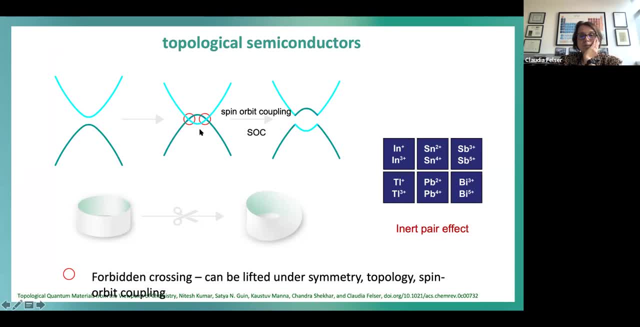 of the bands- and this is also common concept- which we have, for example, in organic reaction, in organic chemistry, and here we have it- simply between the winds and the uh, the conduction band, and this is uh. so it's also was the concept of roald hoffman. he looked for forbidden crossings. 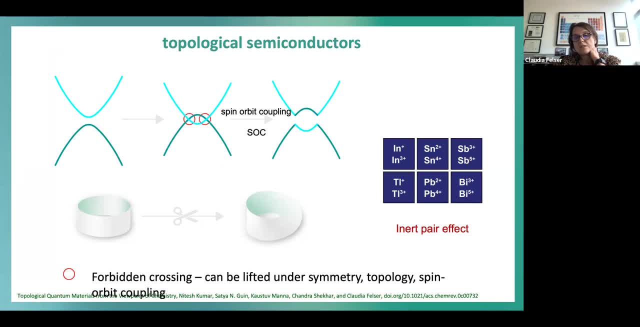 in the electronic structure, in many different crystal structures very systematically and could explain many properties but also many crystal structures here. since we have uh materials, topological materials, we have a large spin orbit coupling we because we like to have heavy elements. so then this crossing is uh forbidden. so we can open up a band gap by 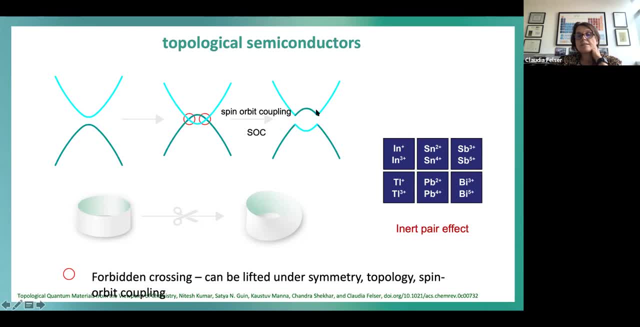 spin orbit coupling and now we have a band structure which has in the conduction band, a part of surveillance band and the part of the conduction band, surveillance band, and while the normal insulators are symbolized, symbolized by a donut, this is symbolized by a 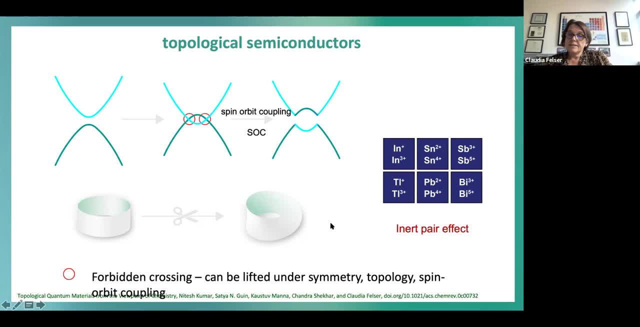 moving stripe. so, um, in the same way like, uh, like we have shown it already in organic molecules. so this is quite happens quite often in heavy elements. so if you go to the periodic table you see a periodic table behind of on my wall. so the heavy elements, like indium, titanium, tin, 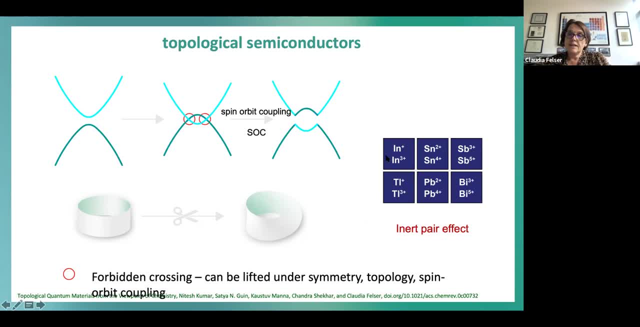 and lead, for example. they are here at the lower part of my periodic table. so the, the indium, is in group three and tin is in the same group. so this is silicon in group four. so this heavy element compounds, uh, they have a different valence compared to the same group elements, which are 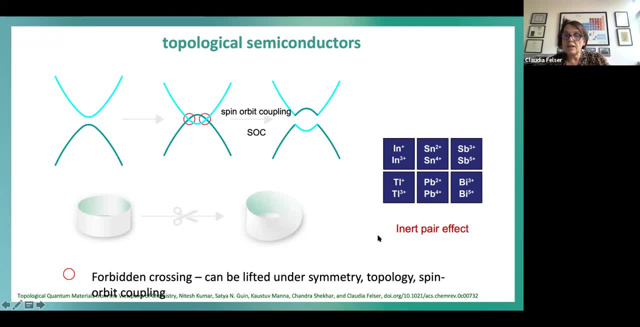 lighter, because here we have the so-called outer s electrons, the five or six s electrons, which are valence electrons. they get because of relativistic effects contracted and therefore the uh, the atoms. to give them away, because they are now very close to the core, is very difficult to ionize them. so 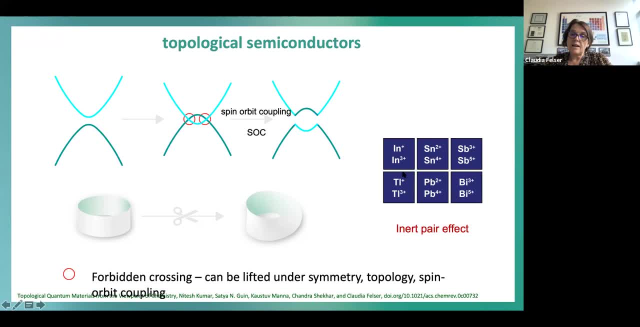 therefore, very often this, uh, this atoms are have a valency which is reduced by the number two, the two s electrons, compared to the lighter elements, and this is the reason this band here is nest band, which comes more or less in this heavy element compounds much easier down in energy and we have 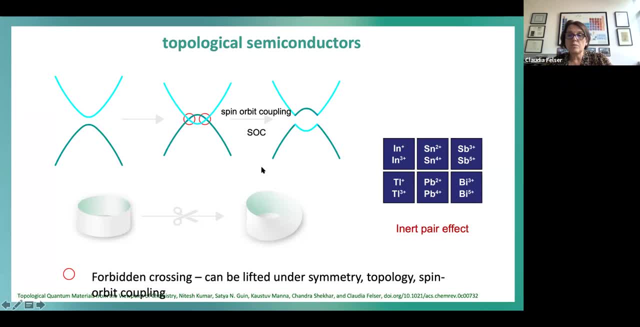 the situation of a forbidden crossing is much more common in this heavy element compound and at the same time spinoid coupling becomes larger. so to find more or less what you, what you learn from quantum chemistry, eventually from Maya and Andre, more or less all the heavy element compounds are topological. 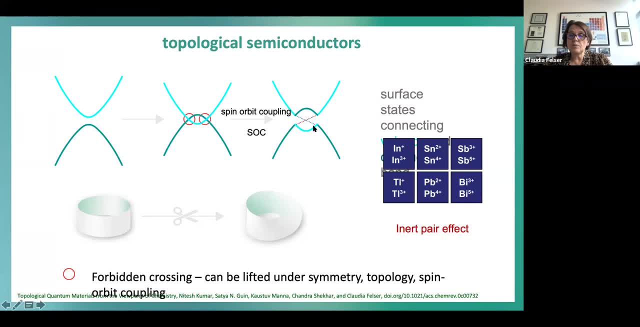 and then if you have this band inversion here, so the conduction band in the valence band and vice versa, so you get new kind of surface states which are uh, which are unfortunately has this little bit uh, which are uh, spin, polarized and uh, here for the 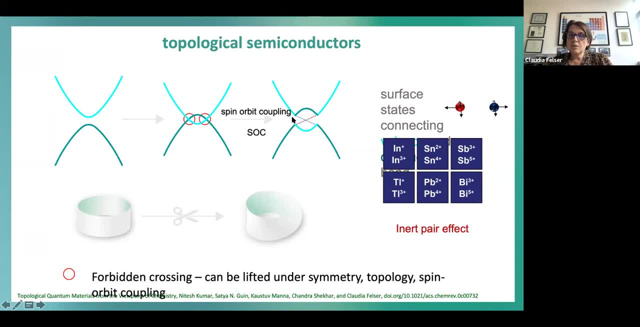 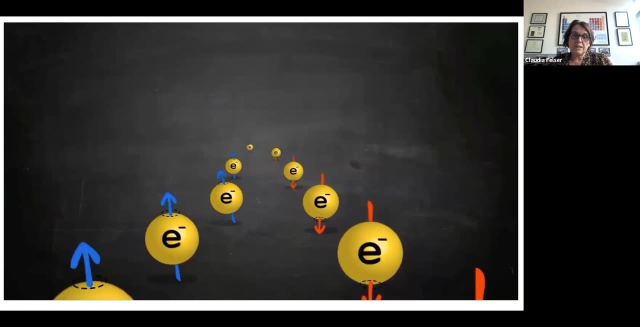 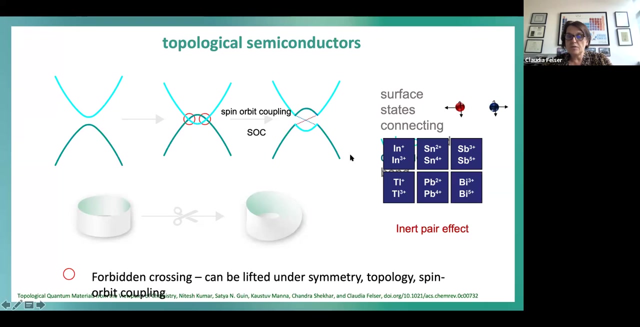 surface states. we have been, uh, momentum locking, so two different uh uh, spin polarization. this are very special surface states which are topologically protected. so, um, here I stole a slide of Maya, so which shows what does it mean if my spin and momentum is locked? but I showed here in the slide. so spin and momentum is locked. related to the 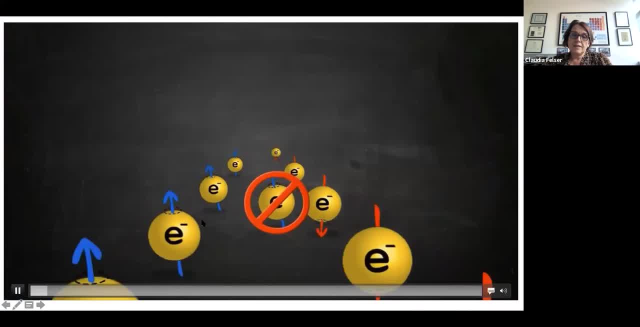 surface state. so it's like uh, so this, uh those, uh, so the electrons, the which are moving. they cannot be easily scattered into the uh electrons of the different spin directions. so they're in this sense protected, and this is a topological protection we like to have. and we see also an experiment if we 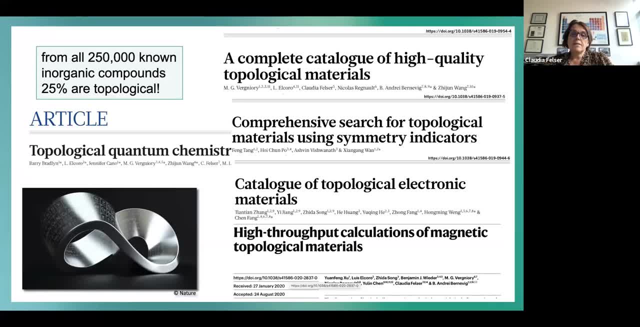 do experiments with this materials. um so, um, so now we uh. the good thing is that all the inorganic uh compounds are in a catalog, so in a database. already the crystal structures- this is uh one where we uh database, where we really are ahead. so if you would have this from all the properties of materials, this would be fantastic. 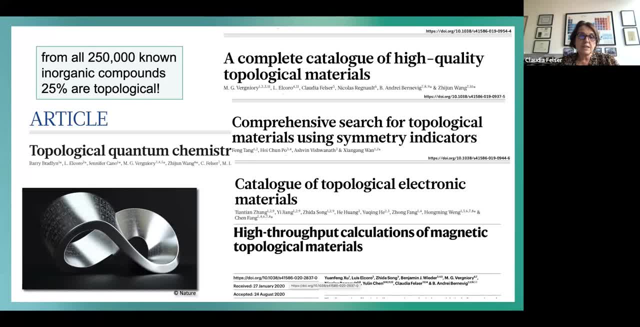 but we have a database with the crystal structure and this could be used. then was used to do this topological quantum chemistry and this has helped to identify all the topological materials and, as I already mentioned, all the heavy element containing compounds, uh, topology, topological uh- if you simply take into account the electrons which are around the Fermi energy. 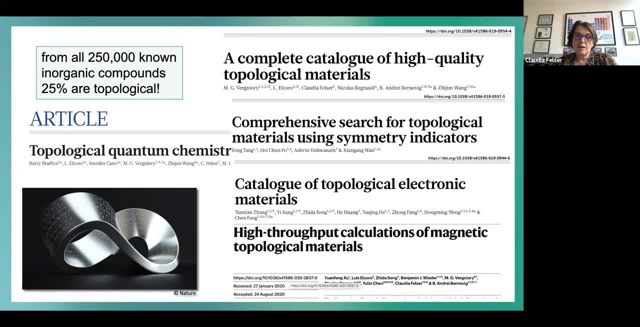 the energy which is exactly the energy which separates uh occupied and unoccupied bands and- and in this sense, if you would allow even doping or uh alloying of the material, we would end even many, many more compounds, because then we could more or less turn nearly every compound into a 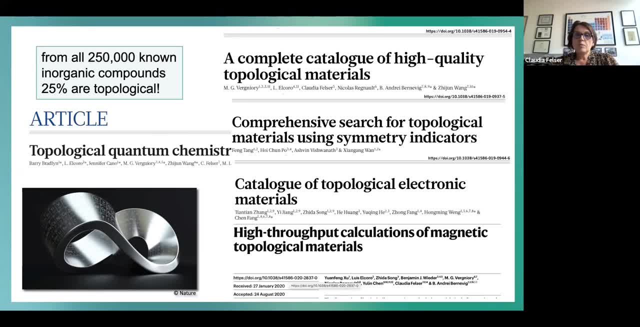 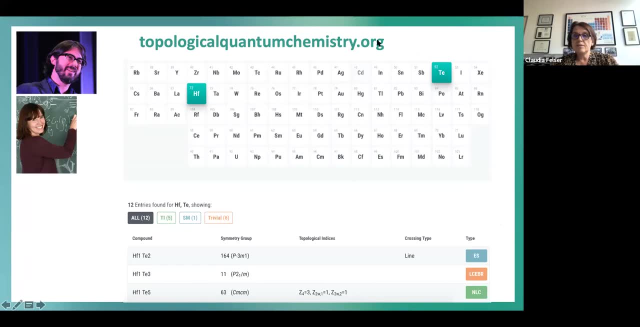 topological material. so this is a totally new design principle and it tells us already that, uh, there are many, many more possibilities to do, uh, to, to, to, okay, so, so there's this fantastic band, uh, uh, this fantastic webpage, so you can even type uh topological chemistryde or fr. you always end. 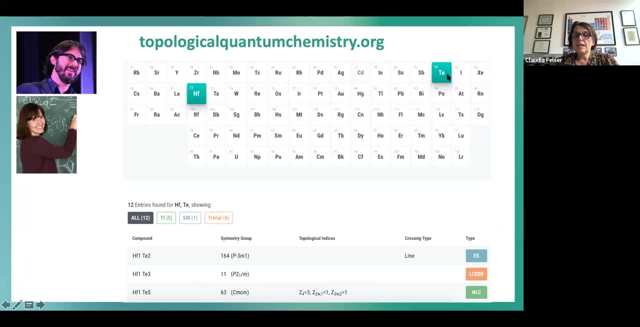 up with this periodic table. here you can click which elements you are interested in. for us it's fantastic. so if you make some new compounds, you simply can more or less- uh, not new compounds, we can more or less check of all the existing compounds, whether they are topological or not. so 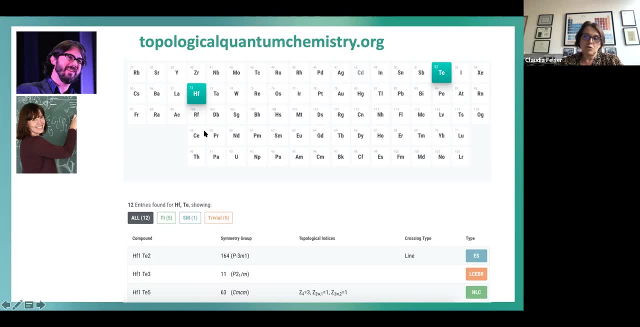 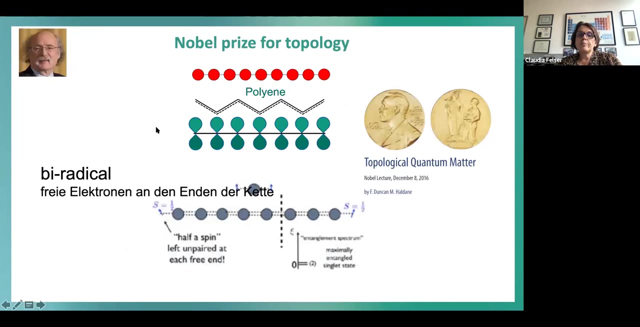 uh, new compounds are still a little bit of change but I'm sure soon, uh, you can even come up with a electronic structure with the position of the atoms and the crystal structure, if you get information whether something is topological or not. so bringing again everything back uh to to, to, to organics and chemistry, to inspire future research in this direction is like 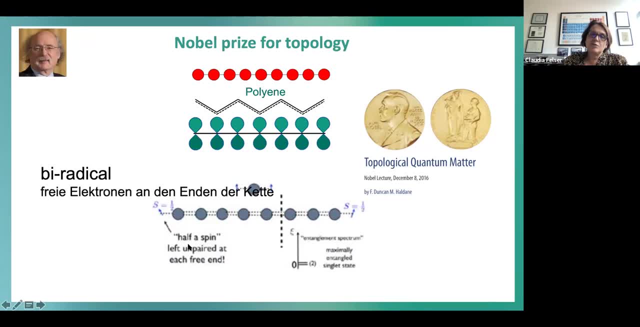 also that even Haldane in his Nobel Prize speech he used uh poly, even double, one single one, double, one single bond as an first example to explain topology. and especially if you cut one double bond and get the radicals at the ends to symbolize the X states here in this. 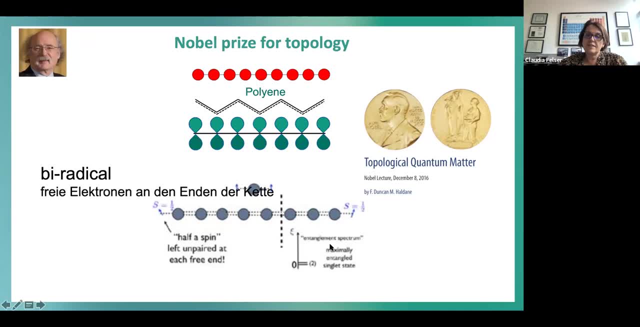 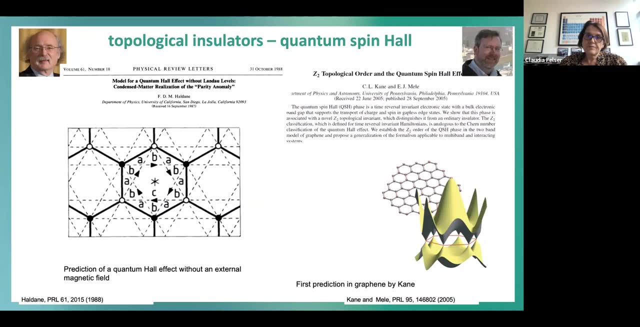 material and I like this very much because it's again shows again the connection between these different fields. so, uh, but uh, for his uh, price winning paper. as far as I understood, this was this paper. he used graphene and graphene again is very interesting and he could show that uh like. 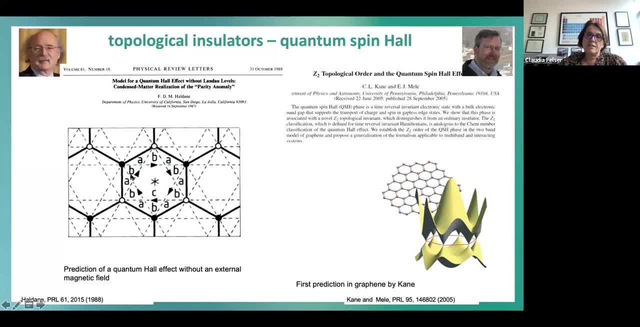 uh what we know, the quantum Hall effect. I shortly will uh talk about this, uh, very briefly also, so you can have even a quantum animal as well. effect. uh, in some materials where you don't apply an external magnetic field, if this material is, for example, intrinsically material, uh magnetic, so this has 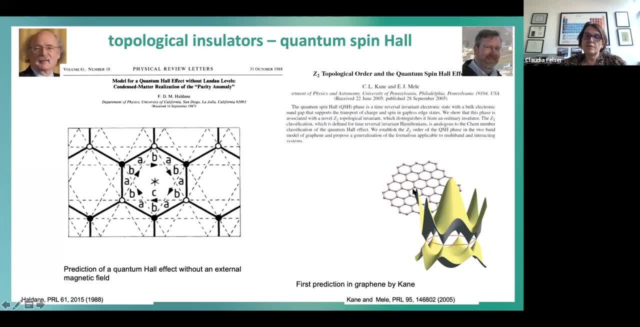 inspired also Kane and Miller to look into the electronic structure of the same material and teeth. they find even that if you have spin orbit coupling, you can use this to have this quantum spin Hall effect, to have this new topological properties. however, if you think about graphene, so the carbon is very light, so spin orbit coupling is very small, so graphene- 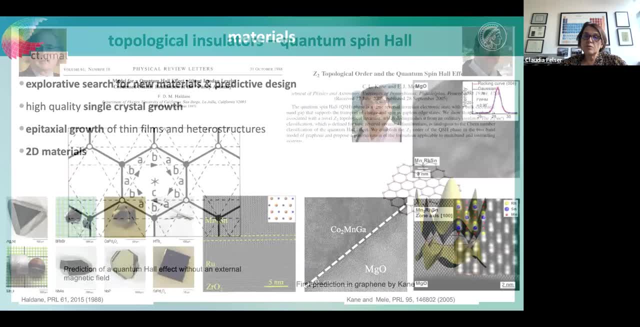 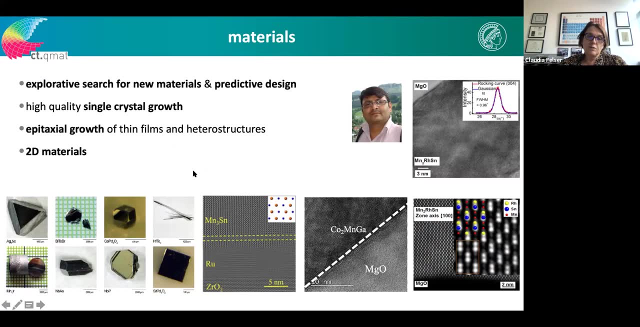 was not the right material and this has inspired and people to look for more materials. so this is a small break where I want to show you so we materials, what are materials in crystal- organic, uh, inorganic crystals- what we are doing and most of the people who are doing the experiment. they nowadays grow very nice. 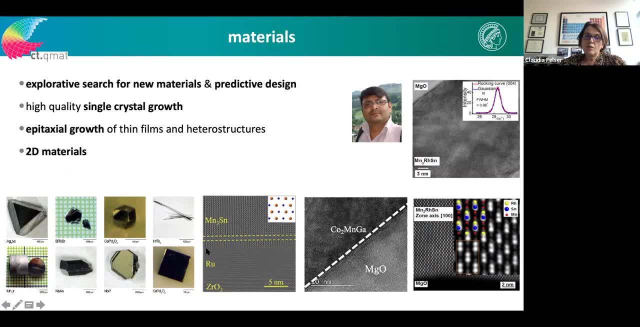 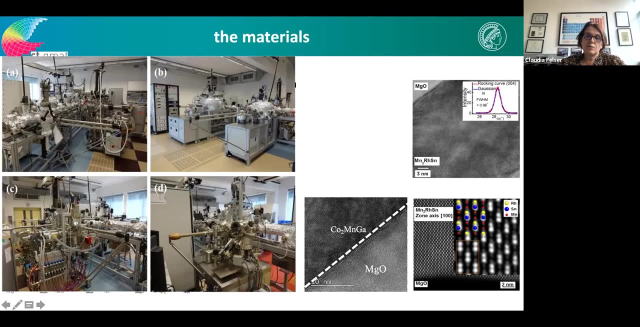 in crystal, which you can see here, is this beautiful examples? or they grow some films to make this new materials and to have this as a basis for investigation, and this is where you do this in film. so you need a lot of heavy equipment to grow this in films. but I think now it's also time. 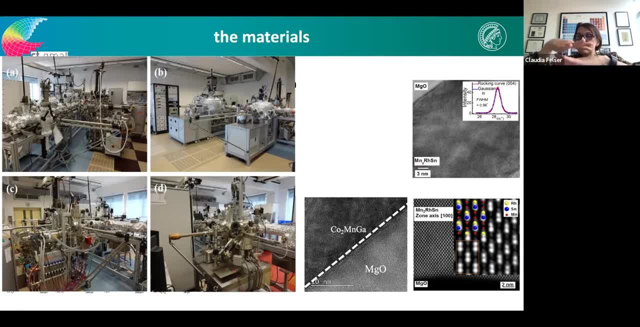 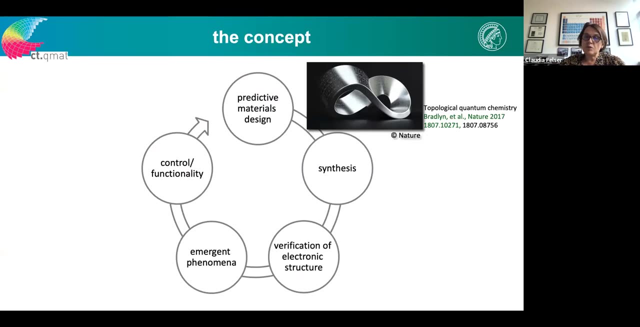 to think more about topology on interfaces. one, yeah, but maybe one can use also the symptom equipment to find more Moray patterns or more interesting twisted material. so what we do after there is this prediction and I showed you. now all the materials are characterized into topological uh materials or not, uh, even magnetic. so we do the 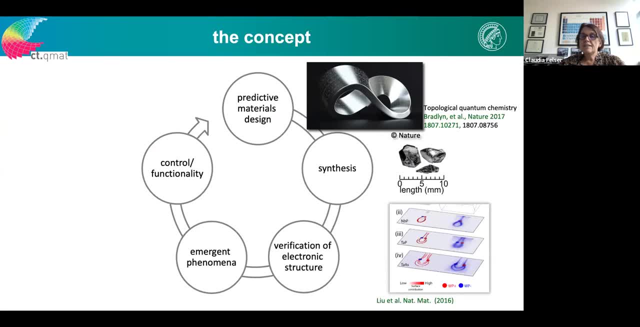 synthesize things, the crystals, what I showed you already, then what we do is like we look at this electronic structure is really the one which we observe. this is the best ways to do: photo emission or STMs, uh uh, investigation. so you can see here the calculated surface states, for example. 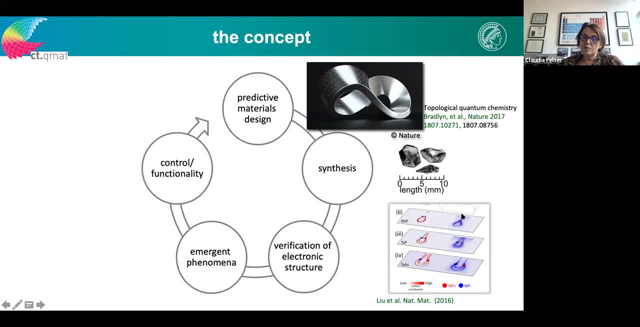 from some vitamin methods. I explain soon what the white semi-metal is. and this is the opposite English software emission data, which shows a very nice agreement. okay, on top we want them to have maybe super interesting properties. the topological material, which shows also super connectivity, and there's a lot of recent work on this mot2 where we found that. 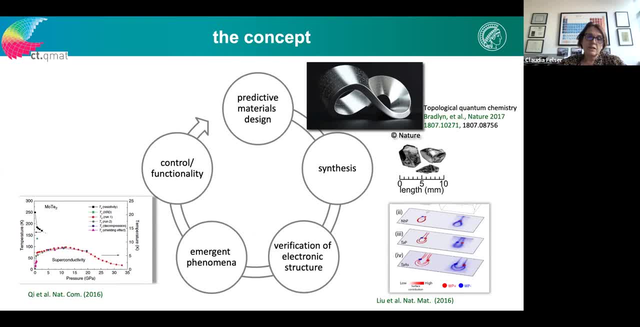 this is a topological right, semi-metal and also superconducting up to uh 10 Kelvin under pressure, and then you want to make at the end, maybe uh uh devices, and this I showed you. we also want to do the prices and people are discussing here, especially in context of uh super connectivity. 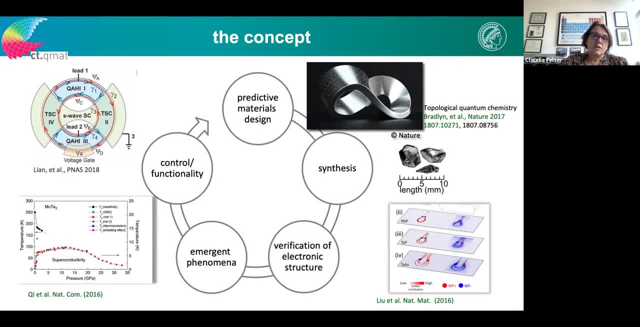 and quantum monomolar soil effect, for example, interfaces. about majorana fermion: so far there's a lot of doubt whether we ever have seen this majoranas, but this tells us, the next generation come up with good concepts where we for sure can find them. okay, so as Maya, uh, as I said already, 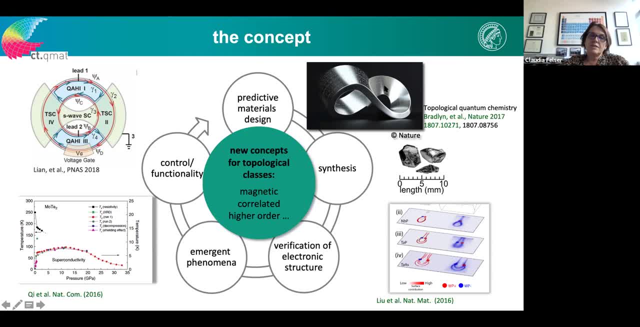 recently there was- even despite- also prediction of all the inorganic compounds using a single particle picture. there there was this prediction of magnetic compounds. so magnetic is done, most of the magnetic materials is done, the space groups are done. so the interesting thing is now to go beyond the single particle picture, and this again for the theoretician. 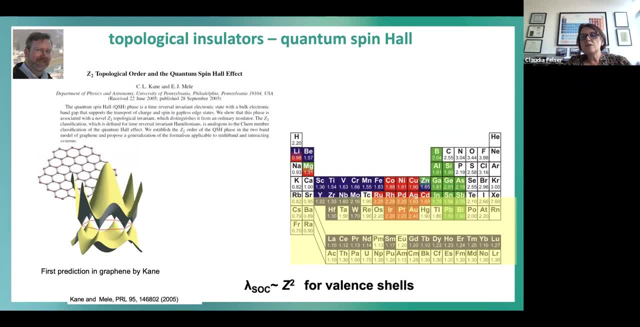 to go into direction of correlation. okay, coming back to a little bit more, back to the history of the materials, history I already told you. so the graphene is too light to show this quantum spin Hall effect. therefore, it was interesting to go to heavier element element compounds, and this is simply to look for the lower part of the periodic. 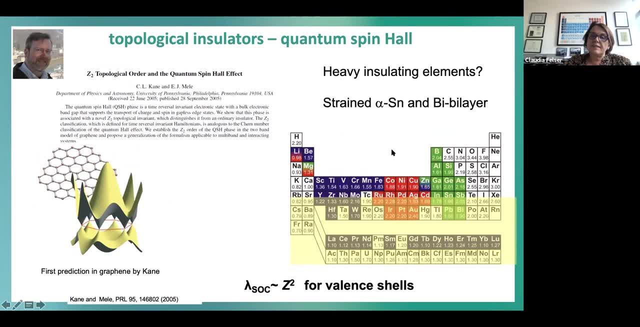 table so far. the first view was that the elements are not the right way to go, because so they are all gases, insulating or metallic, but there are not so many semiconductor which would exactly fulfill the condition. maybe bismuth comes closest to this and tin- here bismuth and 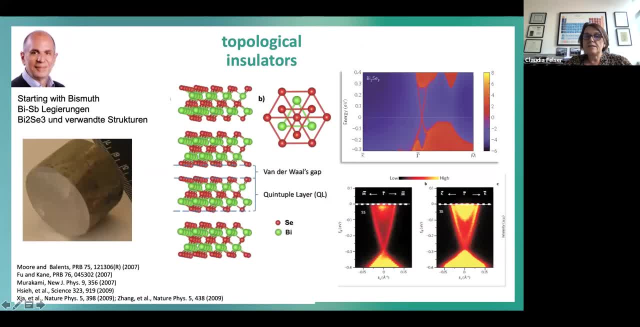 this area are the best materials. but the next idea was to look to binary compounds, and I don't want to spend too much time here, but simply for historical reasons, for the people who are really new in the field. so um so, by starting with bismuth, which is a semi-metal and was not a topological, 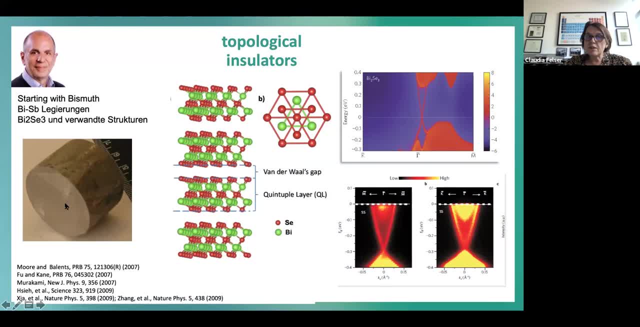 insulator. it was clear that one should look to binary compounds, noise- to find eventually topological insulators. and this is except it has happened here- bismuth, selenite and uh, which has this fantastic surface state, as in the scheme which I told you before, the spin polarized surface State, and this on the experimental. 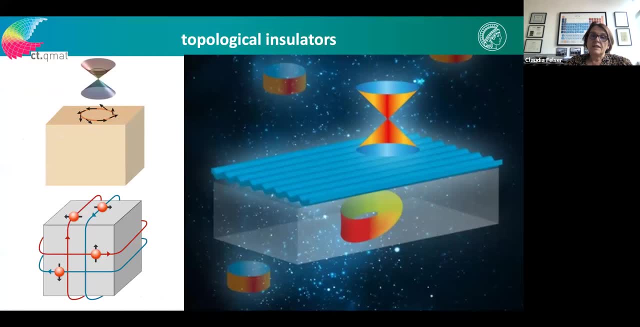 uh, uh, experimental realization. so here we have the example material where we have then this nicely uh spin polarized uh surface State, which you can draw as a picture here, with a nice mobius type intrinsic band structure crystal, and this protected surface state which looked like a Dirac cone. 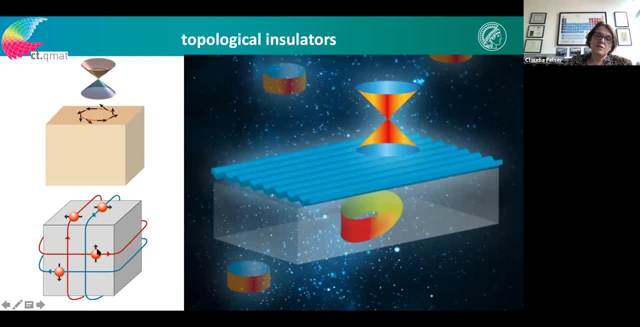 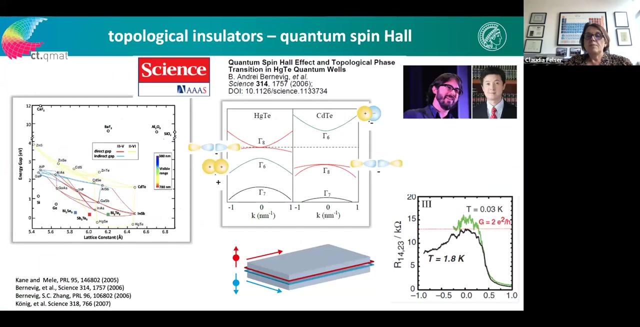 And another picture. we are trying to visualize it this year- like to have this centralized surface state and this material, And the house has been and the momentum is locked at the surface state, Anyway. so this we had already, but you can now do the same, as I mentioned here. 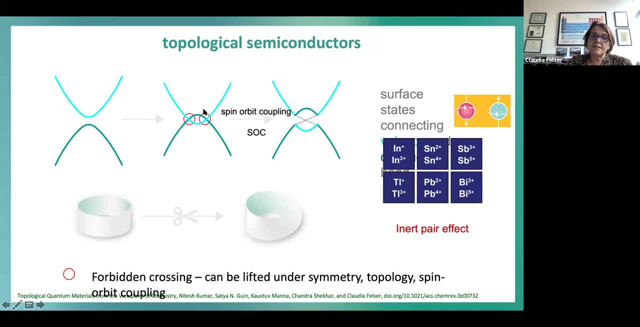 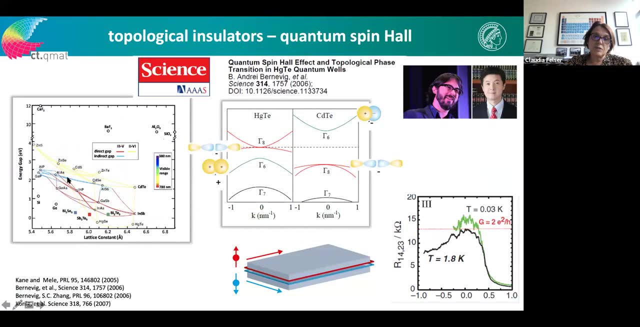 Also looking for some compound which has this overlap between the conduction and the valence band, And people have worked on solar cells since long time. So you see, you can have many binary semiconductors in the range of visible light, but there are. 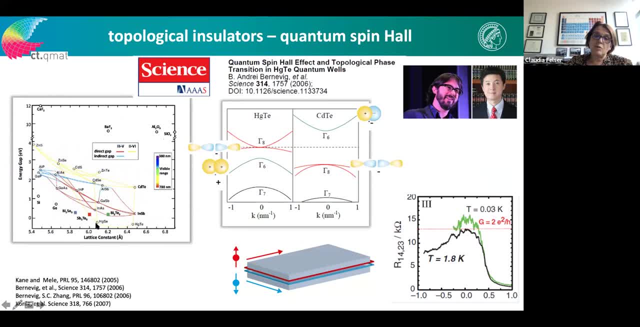 also materials which have a small band gap or a negative band gap, And the negative band gap is exactly what we have here, because we have this overlap, And so therefore, it was very clear. The difference between the two is that the band gap is very small. 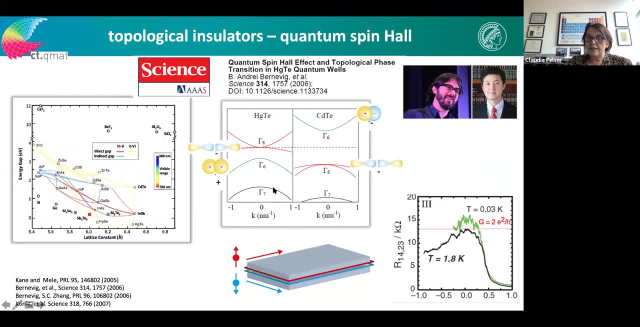 So people look for this negative band gap compound. So, like a normal semiconductor, cadmium telluride, for example, which has a nice band gap, has the S-band here, which I told you comes from the N-pair effect, and the P-band here is: 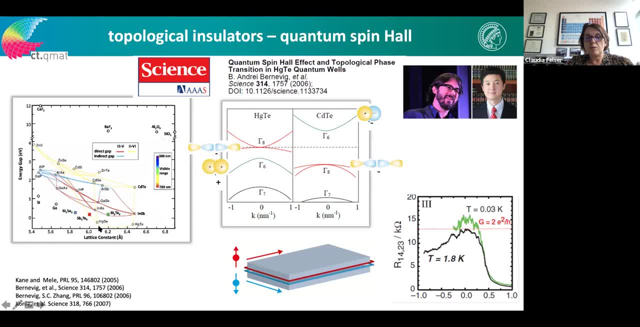 a gamma six and gamma eight band And if you go to the heavier element with the band inversion, macro telluride, you have this band inversion. This was the first realization of the quantum spin Hall effect. but as you can see here, 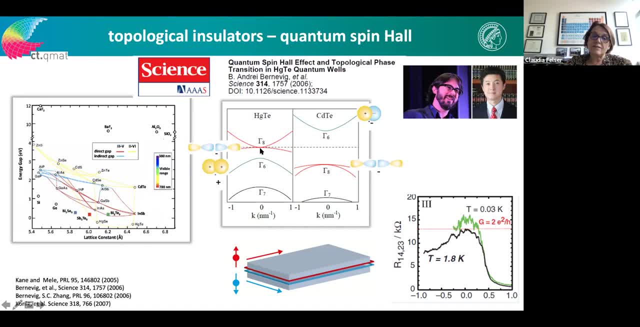 the band inversion leads also to a problem. Macro telluride itself is not a semiconductor. but from semiconductor industry we know that if you combine, if you build this quantum wave structure here, so the synfilms of cadmium telluride and macro telluride, we can build such a quantum wave structure. 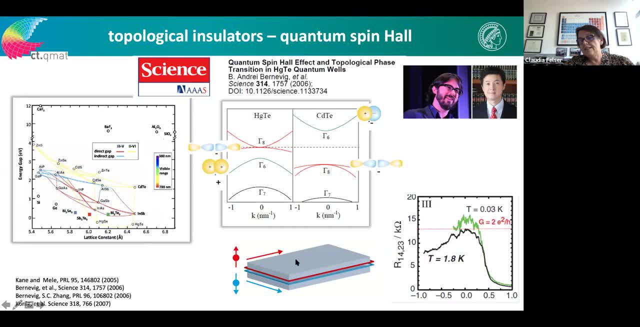 So we get this quantum spin Hall effect, which is exactly. here's a two-dimensional version of a three-dimensional topological insulator. we have this spin polarized Currents here at the edges. Nowadays the plateaus are much nicer. here you see a very lousy plateau. 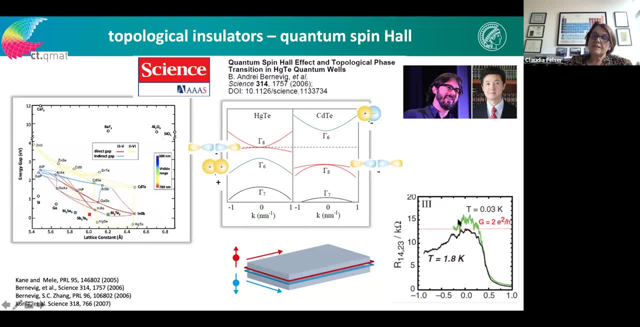 If you have seen the plateaus from the quantum Hall effect, then the quantum spin Hall effect is here, Not so impressive, but this was at the beginning and this has led to a lot of attention, and we already learned about Andrej Brunovic, who is also in charge of quantum chemistry. 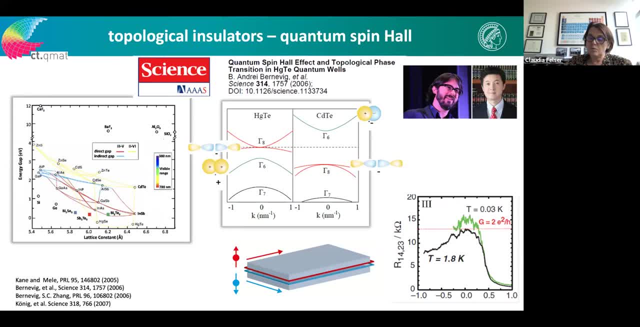 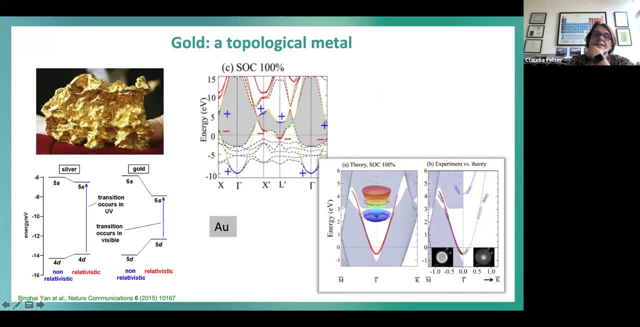 and did also give, I'm sure, nice talks about the twistography. Okay So. So this is a super common phenomenon. it's also shown that more or less the color of gold can be now explained by topology, because you can simply say different from silver. 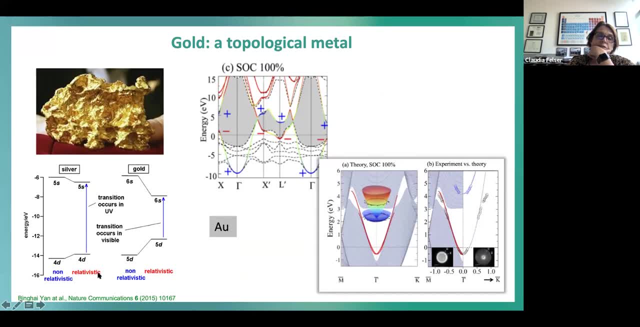 Here you see the schematic electronic structure of silver- non-relativistic versus relativistic- and gold. Here you see that in gold the 6s electrons are much more contracted versus the 5d electrons. Therefore the transition between 5d, 5s electrons, therefore the transition between 5d and 6s. 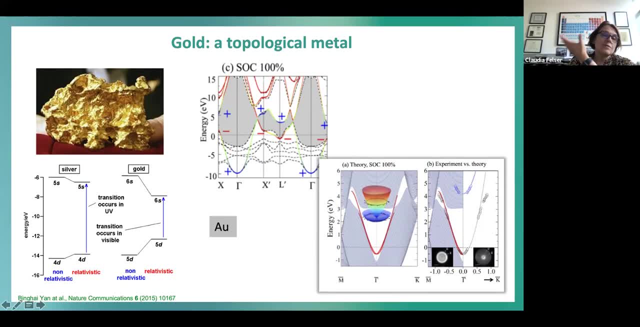 electrons. Here you see that the transition between 5d and 6s is much smaller than in silver, And this is the reason why we like gold much more than silver, because it has a much nicer color. So I like gold very much. 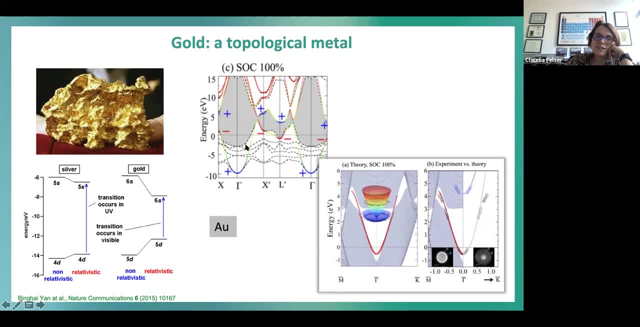 So more than silver. And this is exactly if you see the band structure of gold. this was a nice project with the Bin Hai, so you see that you have here exactly this S-band overlap and the P-band overlap And this is the real band structure of gold. so you see that you have also here a suspended 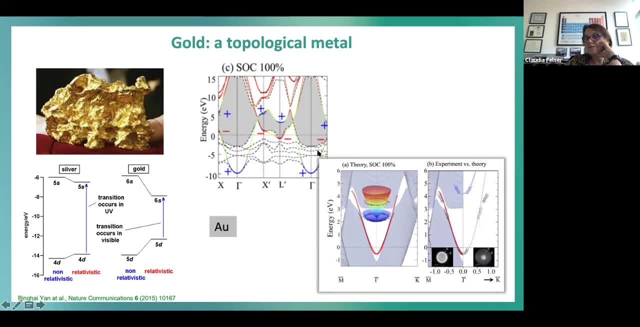 inversion Fermi energy would be a little bit higher. it would be even a topological insulator, So that the surface states are really connecting. the valence and the conduction band was shown here by two-photon electron spectroscopy, because if you see the Fermi 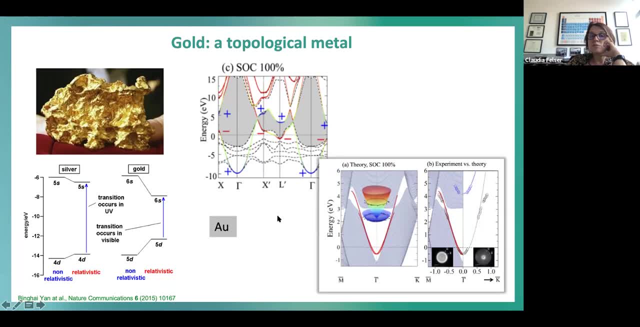 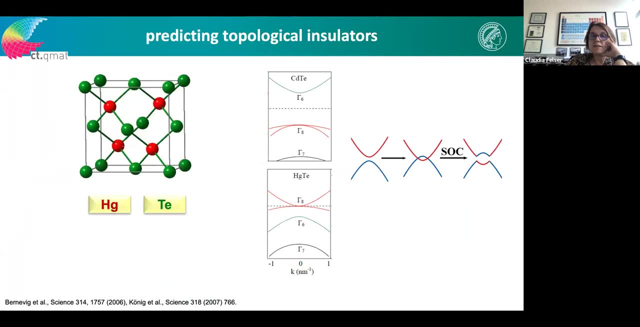 energies. here these are unoccupied bands, so we could really show that gold is a topological metal. So, and I always have to make the bridge to my mostly favorite class of materials. as I said, so, in cadmium telluride the S-band is above the Fermi energy and it's nicely seen that in 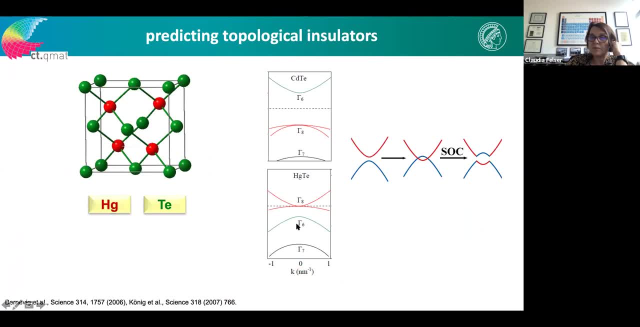 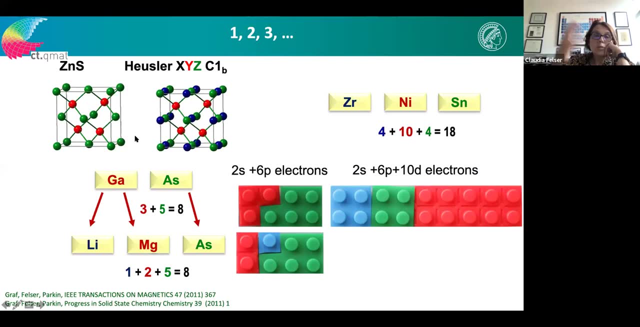 mercury telluride. this S-band comes below the Fermi energy, the gamma six band. so you have this very nice band impression here. so you can find now more materials, and this was a very big event historically. looking then for related materials to the binary semiconductors, Now you can take three elements, four elements. 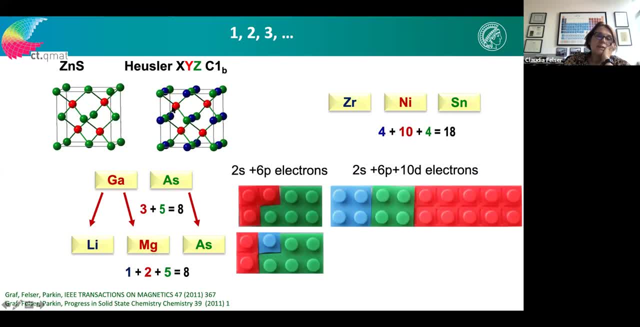 whatever. So if you increase the number of elements, you can make simply the same kind of materials. Here's the example: going from two elements- mercury telluride, for example, mercury sitting telluride- they have all the zinc band structure, the same structure as all. 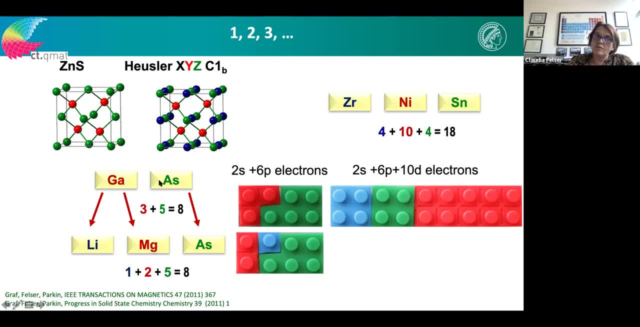 the other binary semiconductors used for solar cells or for electronics like gallium arsenic. So this is a three five semiconductor. so now we could also make them the three elements, and this is a so-called half-oil slug compound, and we can simply have the same electronic structure by 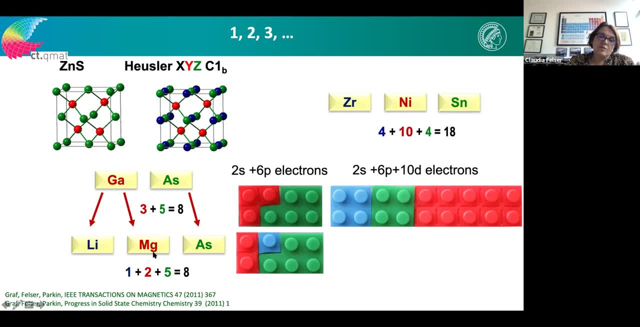 simply re-drifting the electrons over different atoms. So here's like gallium, arsenic, so you can have the same electronic structure like for lithium, magnesium, arsenic because it has the same number of electrons. while gallium has three electrons, lithium and magnesium has also three. 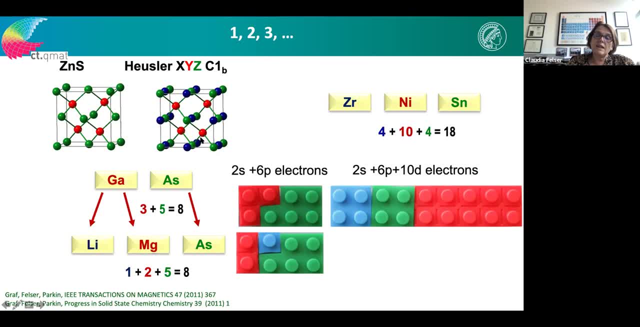 electrons. So this is the reason. Anyway, if we go to three element compound, this has one advantage- and I think we didn't take advantage of all the properties of the Heusler compound- because they have partially also D and F electrons, So we can make semiconductors with 18. 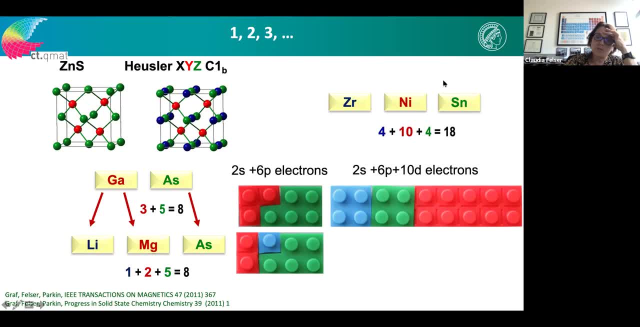 Williams electrons, which leads to much more freedom of redistributing more electrons over three elements, like in the second nickel thinner famous thermoelectric material. and many of the thermoelectric materials are topological, more or less, I would say all of them. 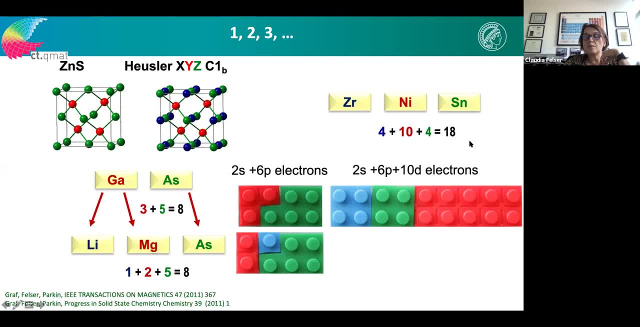 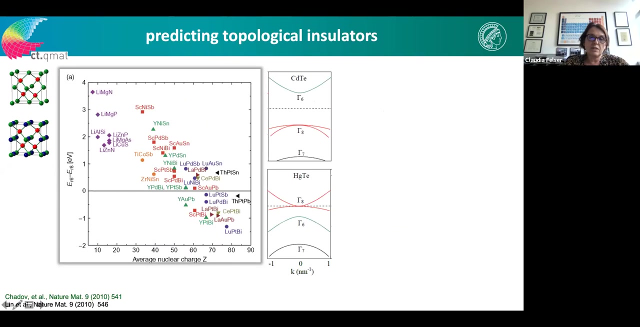 because penorbit coupling is good for thermoelectrics and thermoelectrics really are showing nowadays really again a new promising pathway because they show a very high figure of merit. so this 18 Williams electrons compound, but now you can imagine that I can make the same electronic structure as Mollenkamp. 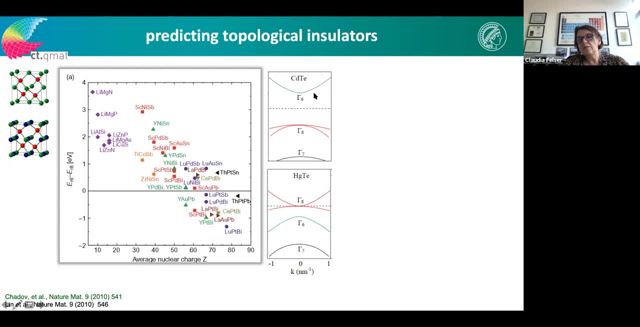 did with this quantum spin hall affecting cadmium telluride and macro telluride, also the three elements. we simply have to rename the compound. so we have many compounds which have the same band structure as cadmium telluride and we have many compounds which have the same structure as 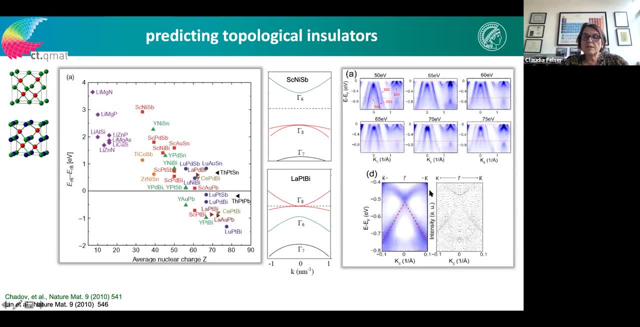 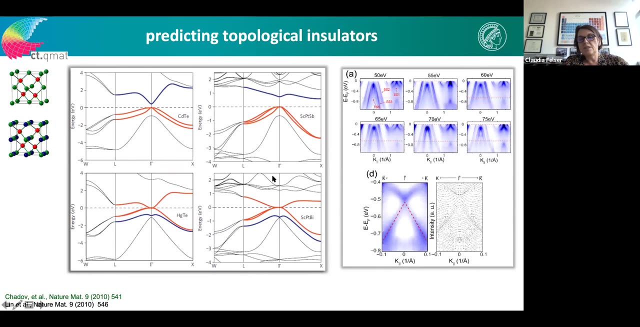 macro telluride. why is this compound interesting? despite of that, they really show this nice direct surface state. they are interesting because here with this ternary compound, we also can have super connect. so this is simply the real band structure, but since i so, which is here in nice agreement, so we have the surface state here, like in macro telluride. 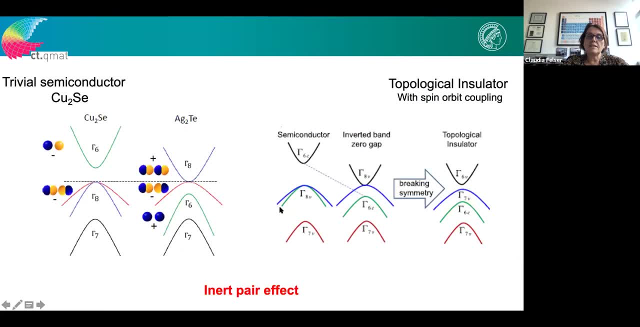 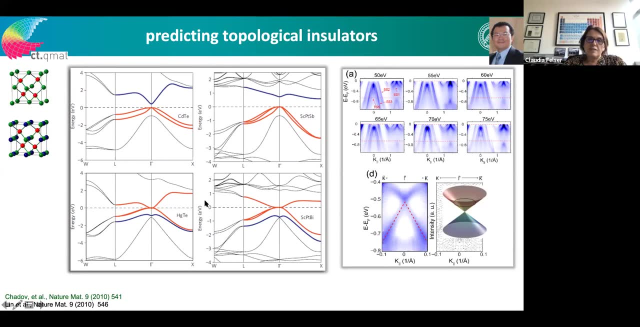 below the fermi energy here in this ternary compound y as a three. oh, now i forgot the slide. but why? as this ternary compounds interesting and i hope that we make some progress now here, because these compounds are also very often superconducting if they have the band inversion. 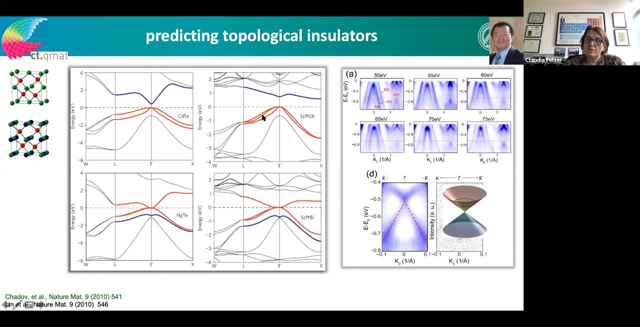 they are semiconducting, for no superconductivity, even if you dope it to uh the same electron carrier, like in the other case. so this is a superconducting and this is a non-superconducting, which might be accidentally- i don't think so- and they are not non-centrosymmetric super connectors. 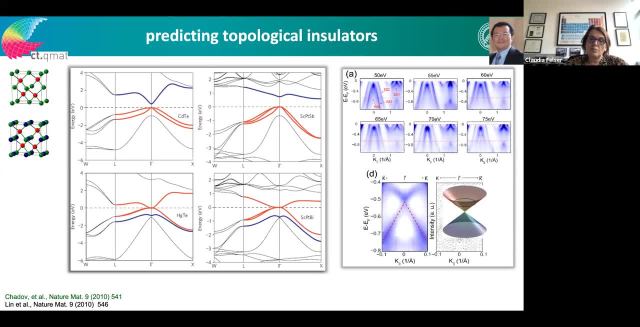 so still, we are working very hard on these compounds to find spin triplet superconductivity in this compound and there is some evidence already. so seeing that, uh again what i said, combining topology, maybe there's a different com? uh properties similar like you saw in twisted graphene. 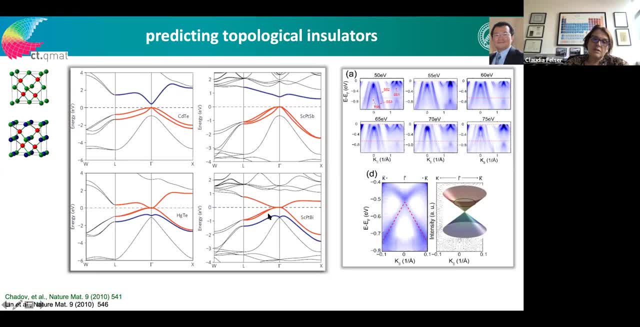 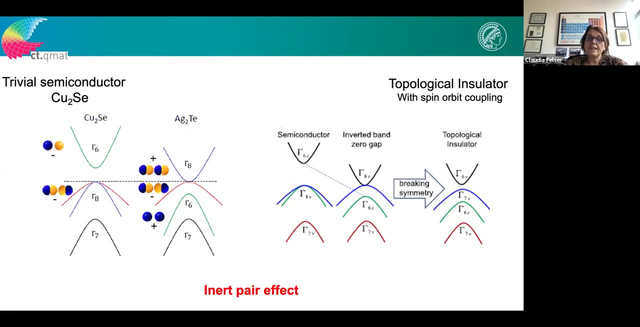 also here you can eventually uh, combine the band inversion with superconductivity. so the fashion is, this is unconventional superconductivity, and then can we go even to more interesting properties, maybe like my rana fermions. anyway, you can find more interesting properties in this compound and i think that's a very interesting question. 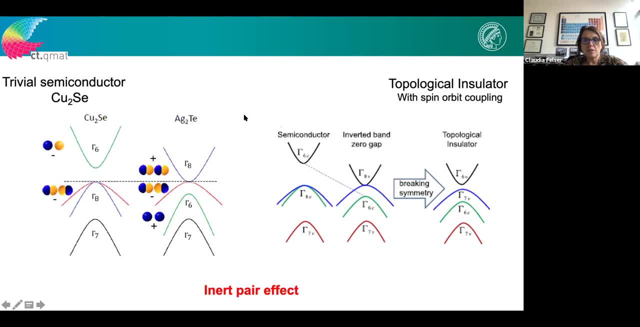 so i'm going to continue and i don't want to continue here because i think i'm. i don't know how long the time for questions is, so that is already, but no questions yet, uh, in the chat. so, since we have here this degeneration of the gamma 8 band, 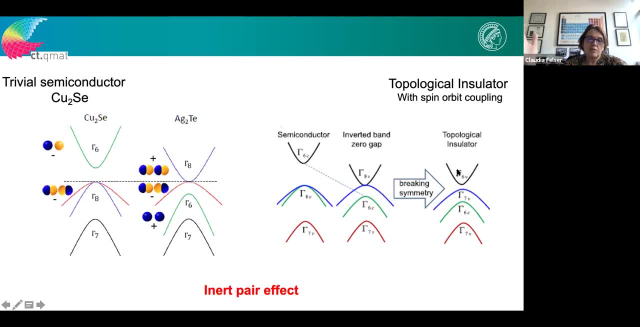 which is not very good. so we can break the symmetry and, uh, make topological insulators here by going to the second question, so we could start with the second question. so what is the final outcome of the machining we are seeing now? what is the total number of electrons? 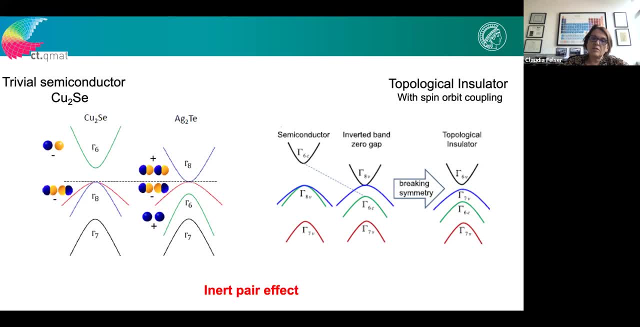 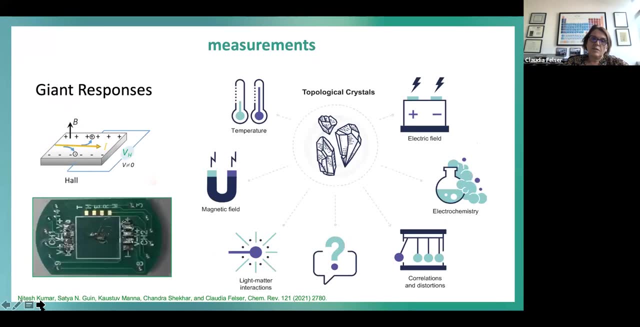 in the clear part of the mass. so let's imagine that you have a JAGenerated co-efficient and so you just give this matrix some mu, virginium silicate, sulfide compounds which are tetragonal direction. i have to skip, eventually, this uh to um hall measurements. so, um, this is what we like to do. 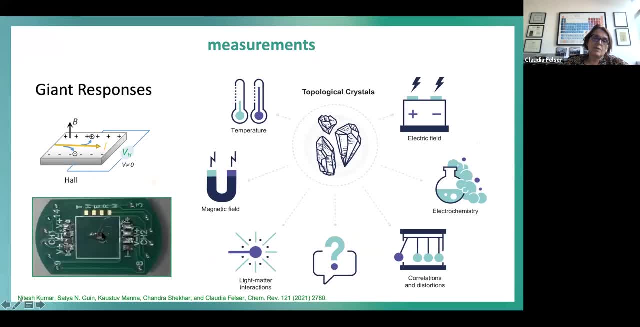 nowadays and maybe go back here. so we like to to measure our uh crystals by hall. so this is the so we we put the crystals, which you have seen before or maybe also this in films, we make contacts here and then we measure the electric current in a magnetic field. this is hard if you 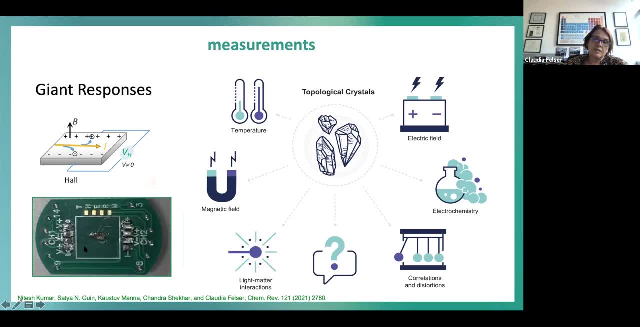 only measure the current, you know whether it's a metal insulator, but if you measure it in a magnetic field, you get much more information. or you can also apply other external stimuli. okay, temperature: we always change the temperature, but we can make measurement of light matter interaction. 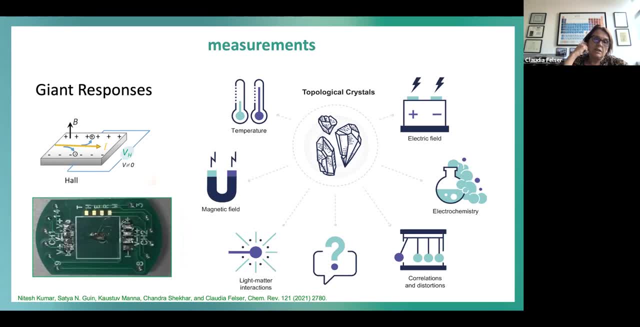 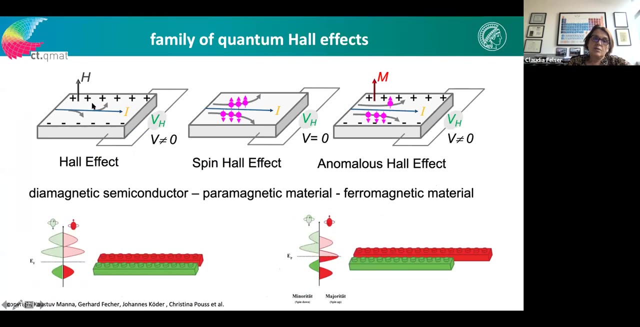 so in most of the experiments we are talking about uh here, and probably also many other experiments, are you build uh, use uh transport measurements. this applied external stimuli, so uh, so. so therefore we can have in macrocellulite, which is the diamagnetic semiconductors and many topological insulators are. 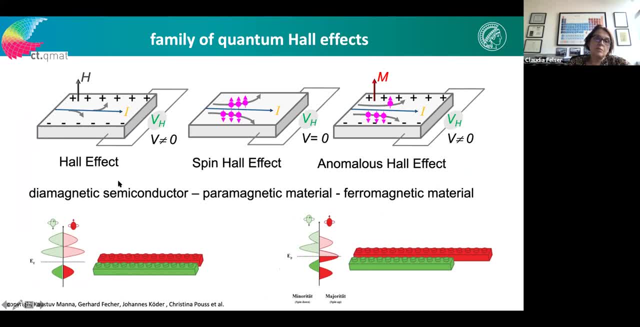 uh insulator, semiconductors and therefore diamagnetic. we measure the hall effect, so we can measure the whole effect. and then we can measure the whole effect and in other plastic, but in our case listed in the, so we can measure. the Elementary robe is a corona. 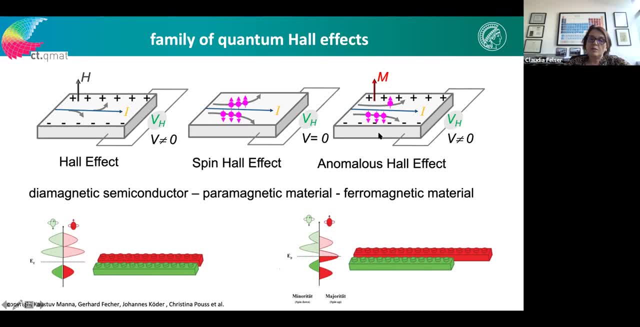 odie material also known as the magnetic material table so that was our first but this what that actually looks like I see �� uh y the For me here the whole effect the anomalous Hall effect this is an additional contribution to the Hall effect coming from the magnetism intrinsic magnetism of the material and then we have the spin Hall effect which is 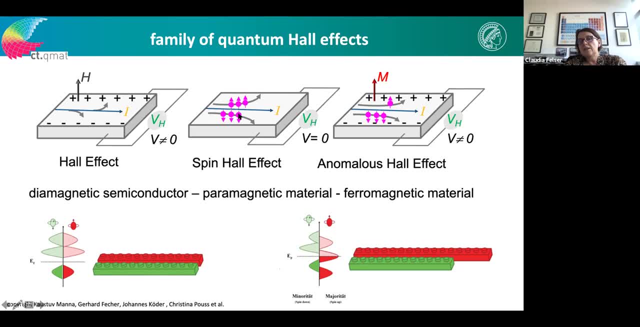 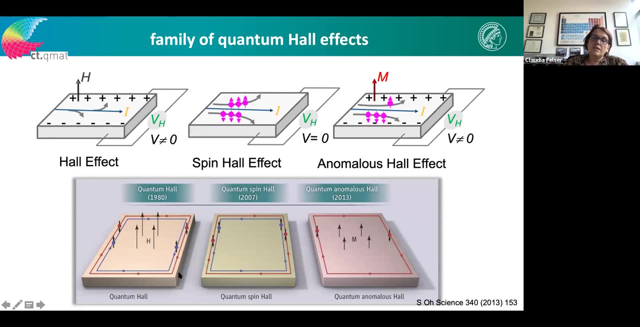 related to in paramagnetic materials, related to the spins in a paramagnet, and this are all classical measurements. the spin Hall effect most of the time is measured with this, with an interface, so. but all this Hall effect has their counterparts, so like the Hall effect has a quantum Hall effect. this is related to the discovery of Klaus von Klitzing. 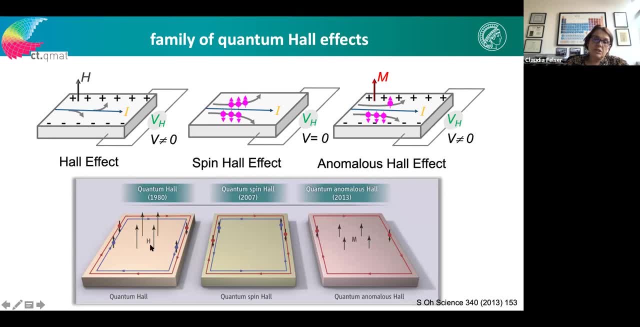 so he took some simple two-dimensional electron gas, again gallium arsenic, very similar like I showed you for von Klitzing, for a more in-campus experiment. for the quantum spin Hall effect looks similar here. you only need a large magnetic field which you have to apply to see this topological. 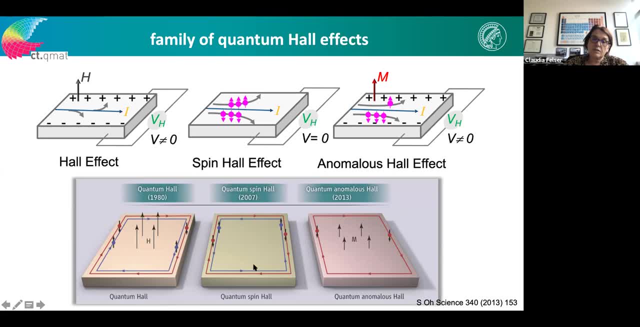 protected edge states, again spin and momentum is locked. we already talked a little bit about the quantum spin Hall effect, where you don't need an external magnetic field, so you get it even without a magnetic field, and then sometime later there was also discovery in magnetic materials similar to the quantum spin Hall effect, simply by doping this magnet. 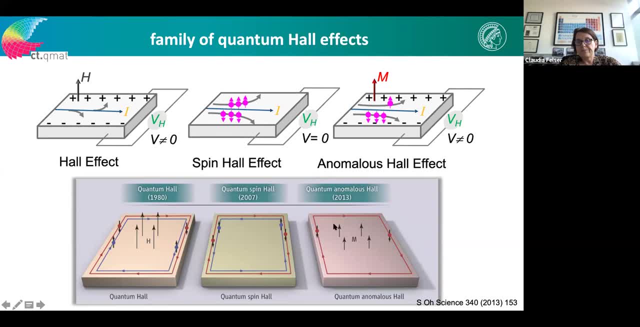 you could see the quantum animal small effect. yeah, yeah, there are a couple of questions. the first one is: how can topology help us understand the preference in nature or elements with certain chirality above the other one? I? this is the. this is the following part. so this is a very good question, Anna. so this is a 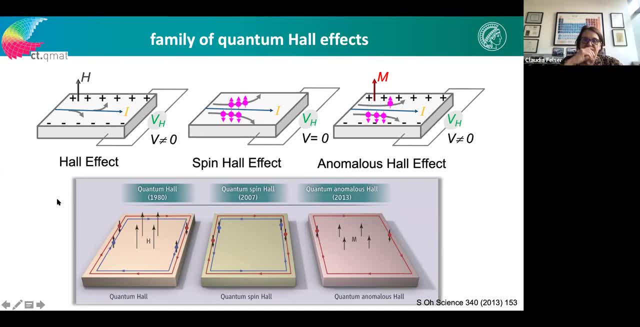 I'm not yet at chirality and I'm not yet at the tribal anomaly, so anyway, so we don't understand it. this is still a big question. okay, so far we don't understand it, but I have some ideas about this and this is the ideas we want to work on. so the question is really: how could it happen that we have 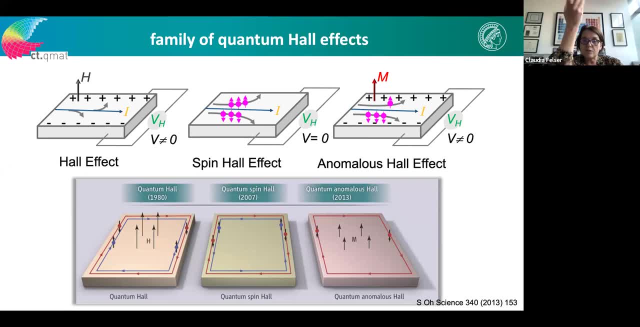 more molecules of this chirality. why are you? we are only molecules of one chirality, so I can simply say I can give you tomorrow a few ideas about this, because I I think today I can talk about the child anomaly, so which will come in the following: 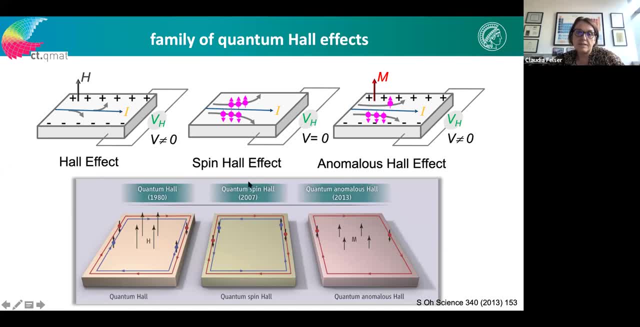 slides. and the second question is also good: does the sample growth rate has any? yeah, Adolfo, you could read. yeah, I can read it. does the sample growth rate have any effect on the final chirality of the compound or are they always racemic? this is also very good question, Anna. so I think they in principle they are so. so this is in solids. 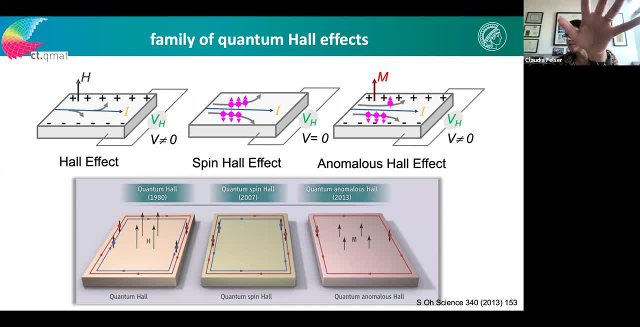 it's not so easy. so so if you look on the quartz crystals which are chiral on earth, you might have exactly 50- 50.. if you do an organic reaction, so you put the molecules in a pot, okay, so you do an organic reaction to get a chiral uh crystal. they are also always racematic: 50- 50.. so the goal of 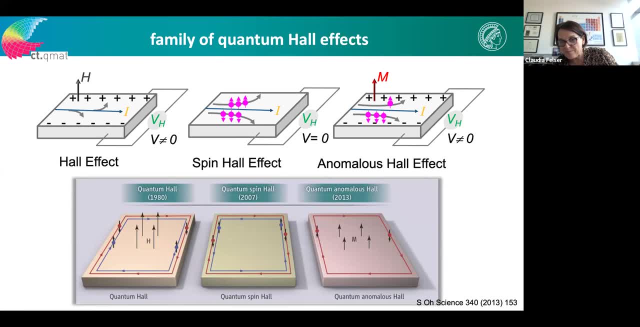 organic chemists is to get 50.01 on one side. okay, then you can amplify eventually and come more to one side. so it's not clear. it's absolutely not clear. but I will discuss a few points also in context of my uh presentation, which is more because I think maybe topology can help us. 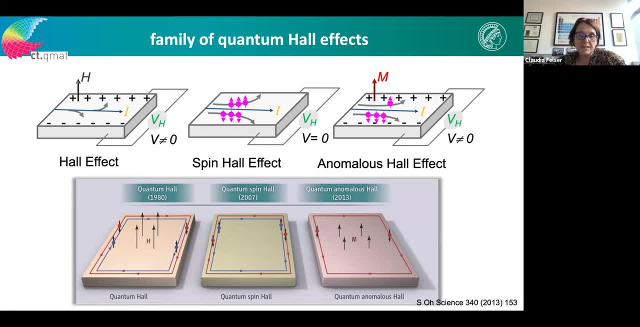 to understand this and also what Adolfo says. so maybe Adolfo should think even more about this to make the bridge between agonizing at one side and amethyst flow end, which actually is non-permanent, overDysłn, astrophysics, high energy physics, topological materials, plus maybe shiver molecules and twisted. 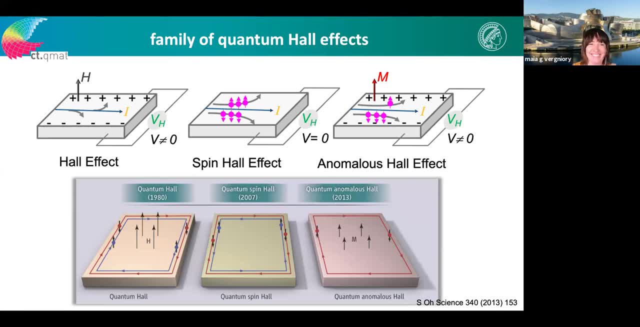 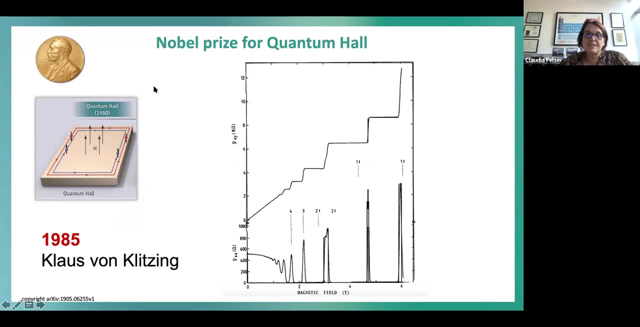 graphene. Okay, nothing less than that, nothing less. So we want to solve all the big questions in physics and biology in one shot? okay, Okay, but in this sense, yes, please continue to ask questions. I still have a little bit of time. Now you stop me, Adolfo. 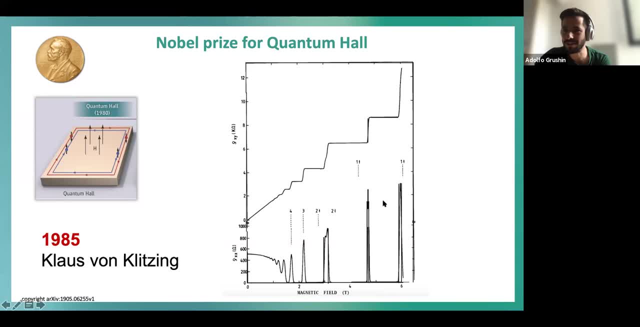 Yeah, you have. like we have 5-10 minutes. Yeah, otherwise I also. so anyway, we can take questions for tomorrow or whatever. Okay, good, So the quantum anomalous Hall effect is what we measure if we measure this very complicated device on from. 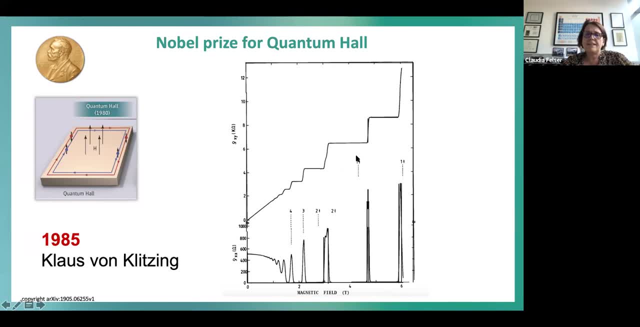 Euclidian. we see these beautiful plateaus. Now you can understand why I was complaining about the Laozi plateaus, the first plateaus from Lorenz-Morenkam. and you see, when you have a plateau, the resistance in the other direction. so in one direction you have a plateau, in the 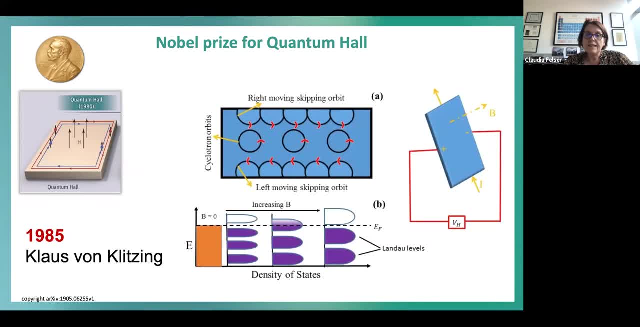 other direction you get the zero resistance, and the explanation is this, I'm sure you know about anyway. so because in the magnetic field- and this is what you need here, large magnetic field- you get these Landau levels and if you-. 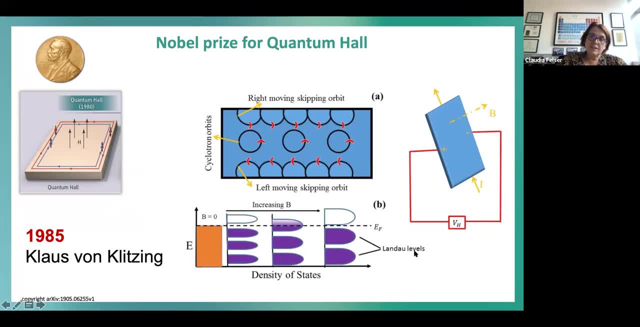 have only one Landau level and this Landau level depends on the magnetic field. And if you only have one Landau level below the Fermi energy, so all electrons and the zero Landau level, if you have more, you'll see these plateaus, more plateaus. 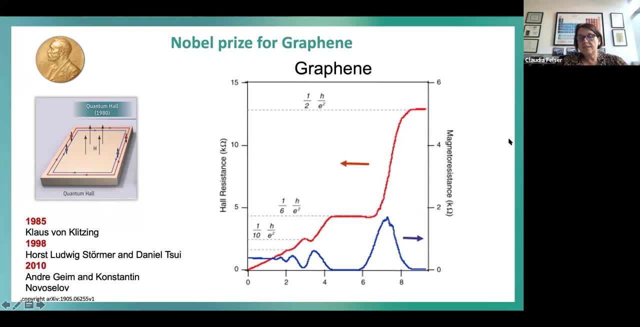 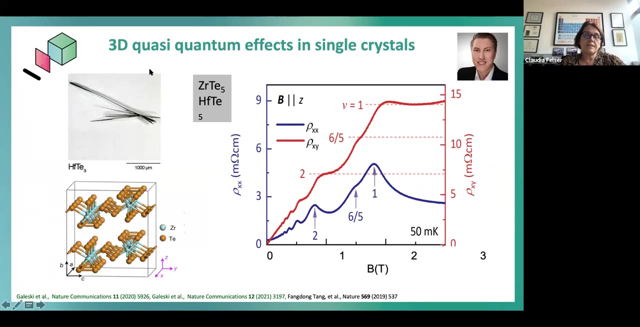 Anyway, what you can see, even in graphene at room temperature- And you see also this: fractional values. I don't know whether I've shown it, But for me what's very surprising is that what is new is that you can see it even nowadays. 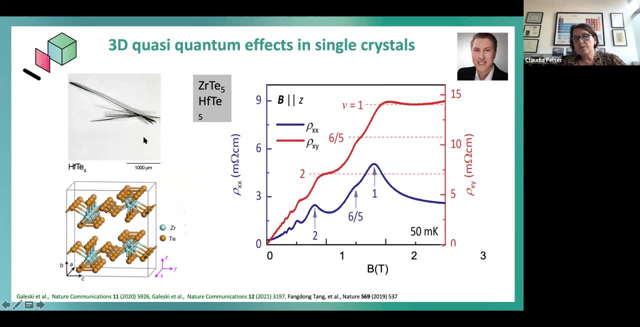 in single crystals. So this is another interesting open area where Johannes is working on also. So can we have a 3D quantum Hall effect in single crystals? How do we have to design the single crystals? And he even saw some fractional quantum Hall values. 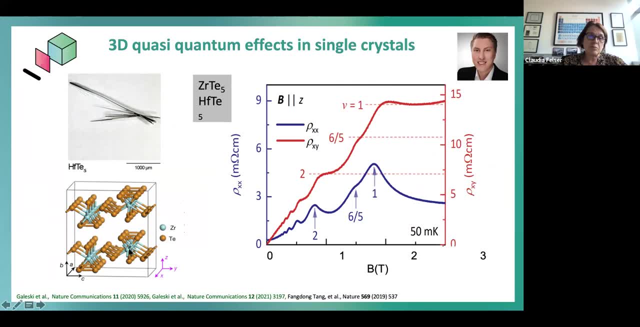 So I always say, if we would have better low temperature, better measurement at lower temperature earlier, so we would have maybe even found the quantum Hall effect earlier in single crystals. This is the cronium telluride and hafnium telluride. 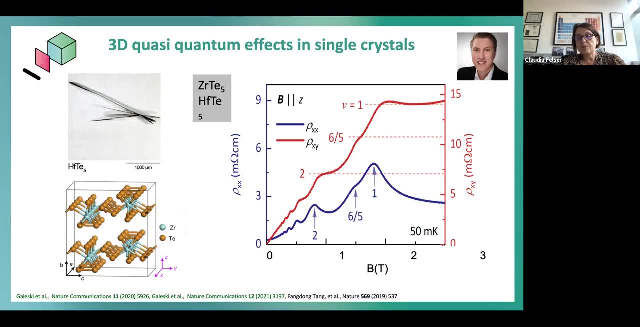 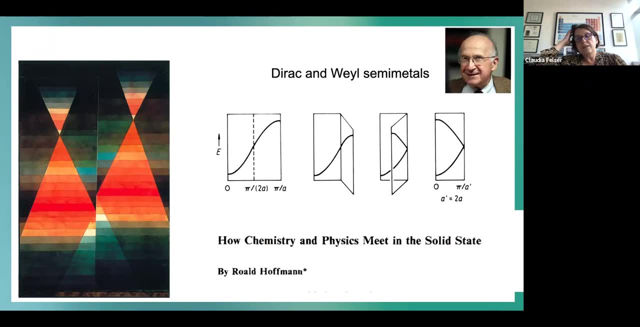 And we didn't need to wait until we have these very defined samples from Klitzing had, which enabled him to find the quantum Hall effect. OK, So, anyway. so, going then back to Roy Toffman and what he taught us despite of all looking. 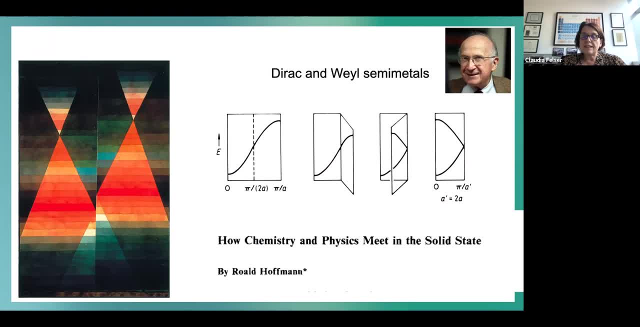 for the forbidden crossing, et cetera, is also if you have one atom in the unit cell and if you would have one hydrogen atom or one S-electron in the unit cell, you would have this very simple Venn structure, which is parabola. 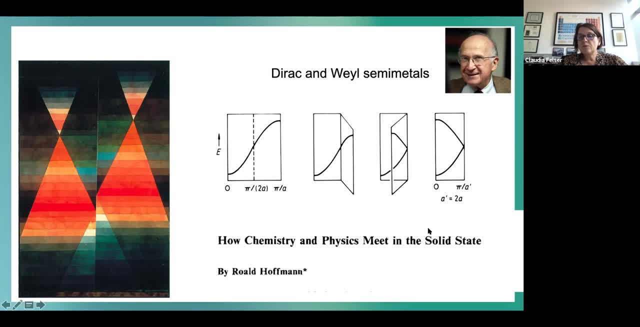 But in the moment when you have more atoms in the unit cell, your unit cell is doubled. So in reciprocal space my bryan zone is halved. So we fold down the Venn structure and then we end up with this. This is a picture from this book from Roy Toffman. 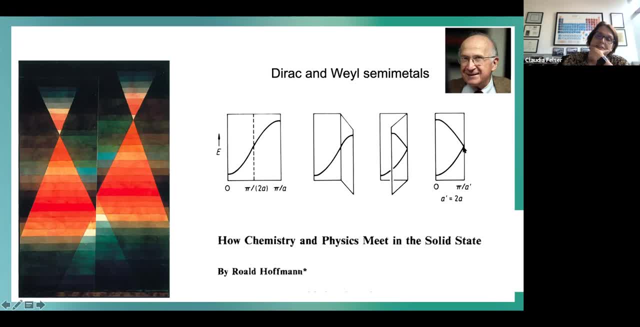 And we end up with this linear dispersion at the edges of the bryan zone here, And this is what we exactly call a Dirac cone. This is a picture from Paul Clay Here very nicely showing even two Dirac cones, white semimetals, which he already had in mind. 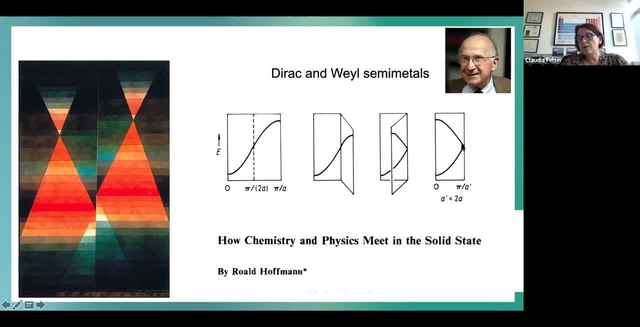 And so this is also why this is not very uncommon. So crossing points, which this linear dispersion in the Venn structure, Like we, like in graphene- and you heard a lot about graphene- is also quite common because it's the simple features of Venn structures. 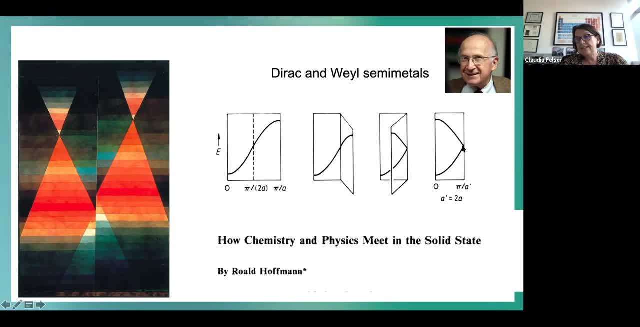 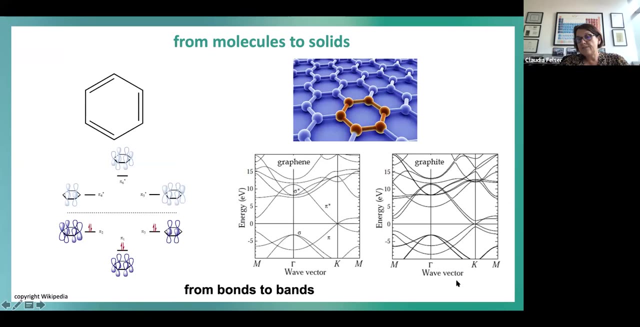 The question is, is the Fermi energy heat exactly here? to see the nice properties in transport, And this is very nicely in a simple Venn structure, really exactly in graphene, As you can see here in graphite. you already saw, see that even in the original three-dimensional case. 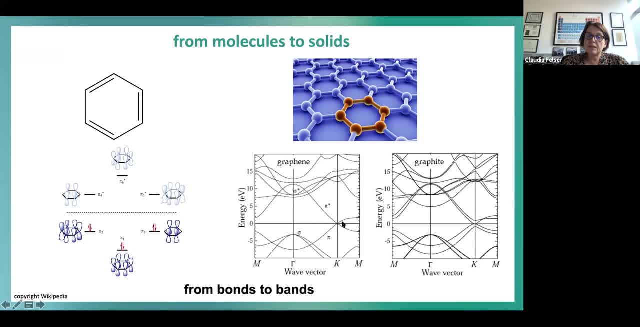 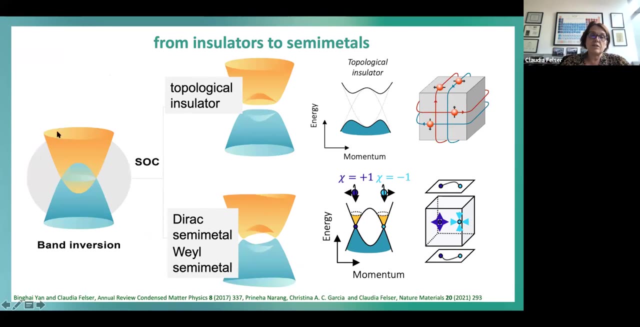 Venn structure is not so different, But if you go to graphene it becomes really nicely linear And this is related to the unusual electronic structure of graphene. So we like this linear Venn dispersion And here again the three-dimensional picture. 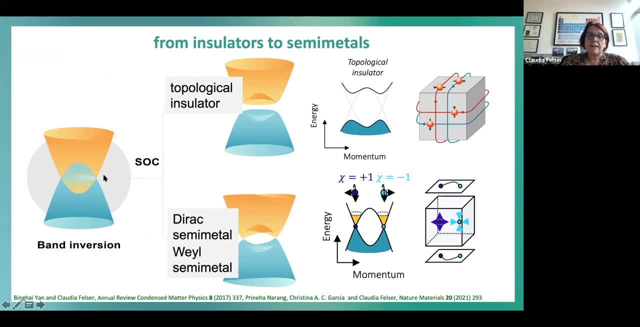 of our overlap between the conduction and the valence band and the overlapping area which is the line here, for example the nodal line. Then if we have a spin-orbit coupling, we can have topological insulators, as we already discussed. 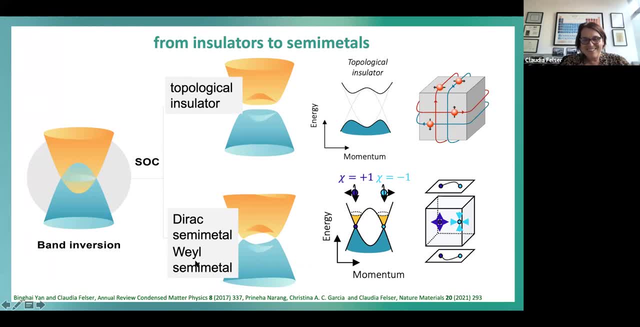 This picture looks normally different, but it's simply OK. Sometimes it happens. Or if we have points in the Bryan zone, like here, where we have points which are protected by symmetry, by a chiral, by rotation symmetry, for example. 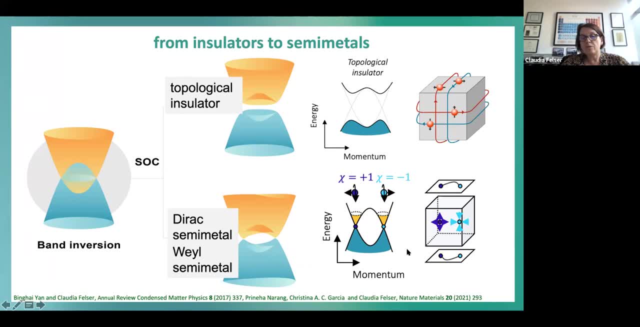 then we might end up with this linear dispersion, as I showed you before, which is also if you have back-folding up Of electrons, So of the back-folding of the Venn structure, Anyway. so if you have these crossing points, 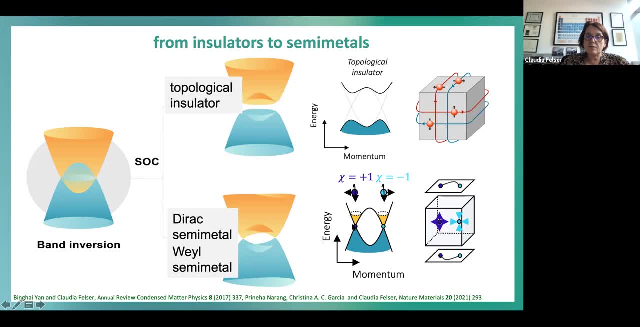 like here in the Bryan zone. so these protected points. So this is again interesting because then we have the same remetal And depending from where these points are- on high-symmetry points or on low-symmetry points- 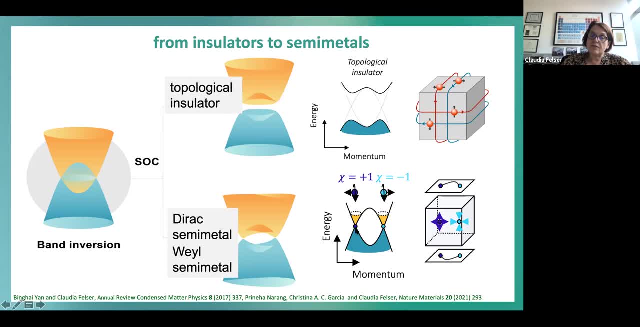 they can be in low-symmetry points. We even can have a chirality here, which means that if we have it in the high-symmetry points, these points are falling together and are degenerated, But if it's on low-symmetry points, 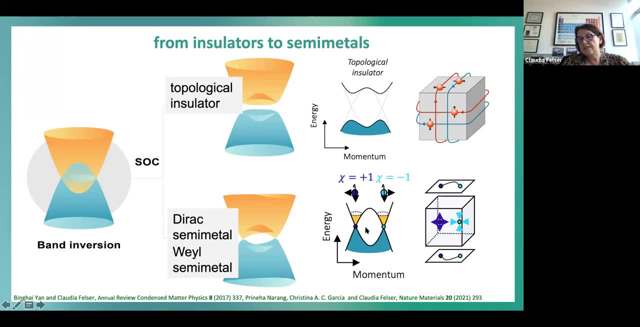 or if you apply magnetic field, so these points, the degeneration is lift, So they have a phase, So the spin and the momentum which is locked on the electrons, so they have different chirality. So this is again. so before we talked. 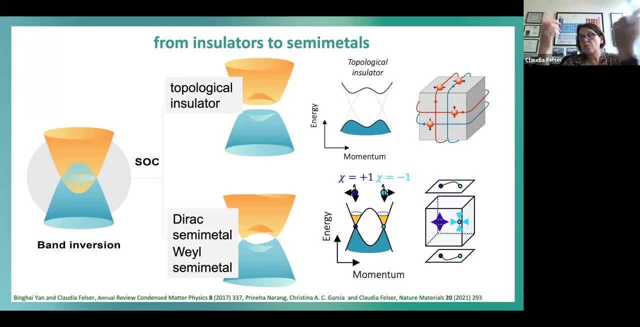 about chirality of twisted graphene. we talked about chirality of molecules, But here we talked about chirality of electrons. So in the moment when the spin and the momentum lock, we can talk about chirality of the electrons, And this makes this super interesting. 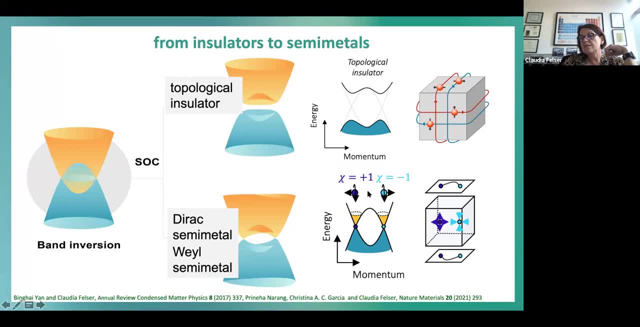 because now we have similar likes, the chirality of molecules, the chirality of electrons, And this can lead to very special properties here, like you maybe already know as a theoretician. So we can have. it's not as nice as it should look here. 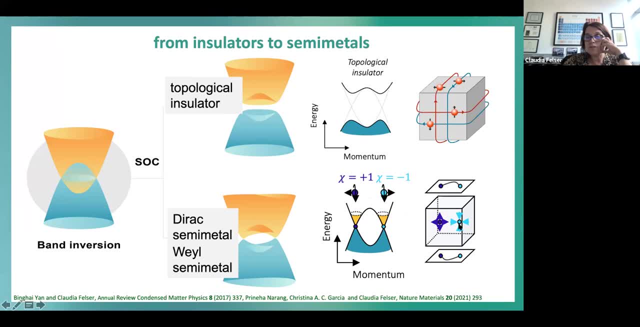 So we have this In the bike electronic structure of this material, we have this y-point, so-called y-points, which act like monopoles. So we have, because of the different chirality, we have also different properties of the baryphase. 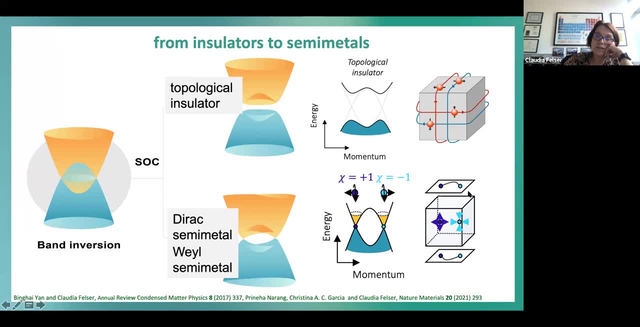 And this leads also to this Fermi arcane surface states. And this is what I think is super exciting, because so now, having chirality in crystal, chirality in molecule, chirality in graphene, just graphene, and chirality in electrons, Why is this so interesting? 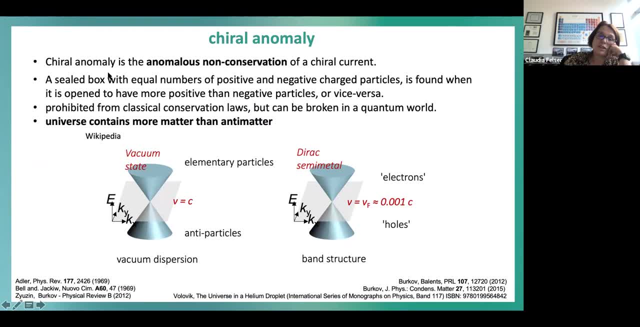 Because for white semi-metals there is this very nice prediction of the chiral anomaly. maybe boring now for Adolfo, but super exciting for me because this is even described nicely in the Wikipedia, because this is a concept which comes even from high energy. 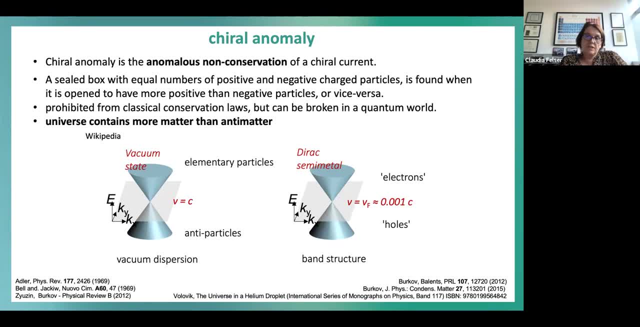 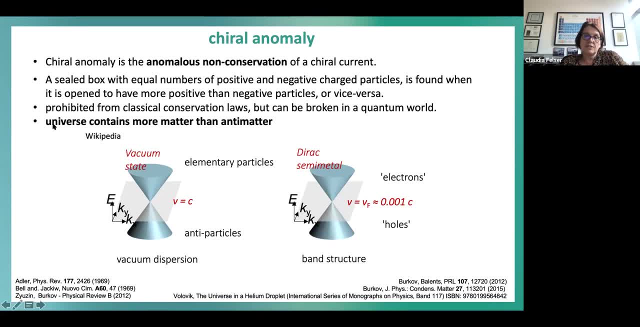 If you have to take into account relativistic effects and and high energy physics. they do the same as in solid and then high energy physics they try to understand the asymmetry between matter and antimatter and fluctuation of the vacuum state and their speed of light. the speed is the speed of light. 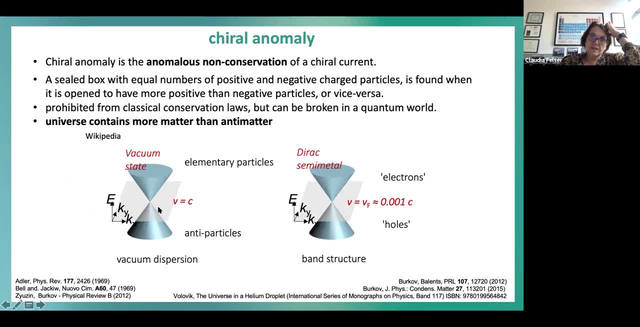 But they have the same same description like we would have and we have here only in our semi-metals, electrons and holes and family velocity. but the same is the case and the child anomaly is in high energy physics, this one possibility to understand maybe the asymmetry of light. 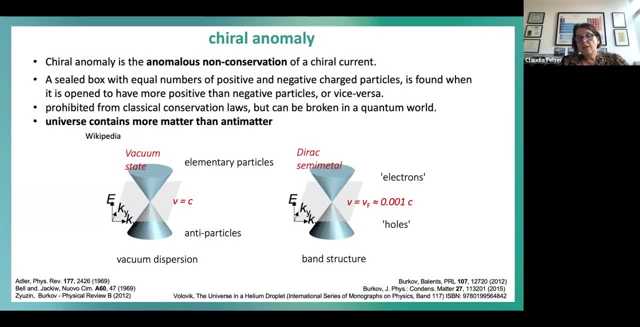 matter and anti matter. so far it's not proven experimentally or some high energy physics, but still people doing experiments, for example nowaday on BR, heavy iron collision. they try to show this asymmetry and therefore it was very nice man. it could have been by similar. 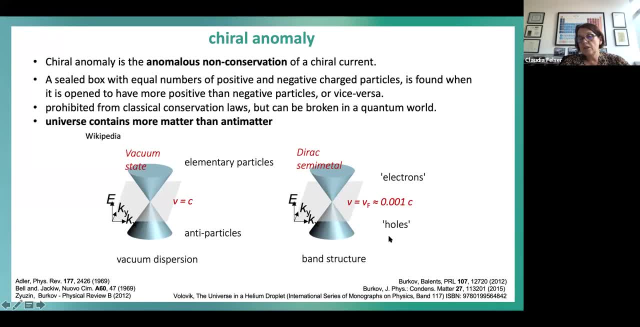 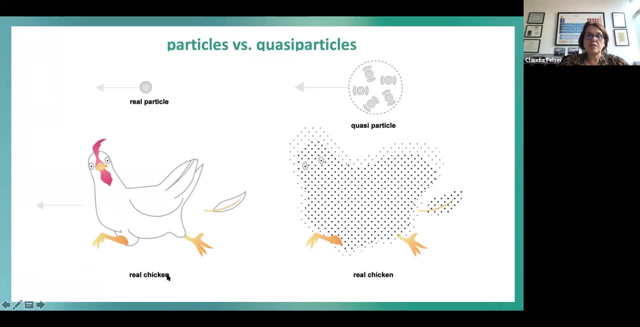 methods were discovered that invites him, a method we maybe could show as a, as a quantum simulation that we can have eventually this child on my, But he will be more talk about. this is a nice picture from your hand: stone. more about quasi particles we be. 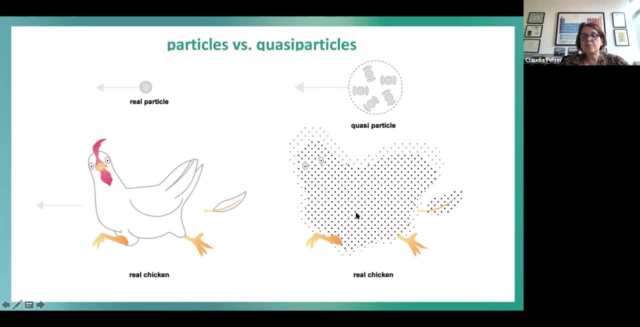 In solid, so because our particles get dressed, but it's not like the rich chicken, but it still looks like the real chicken and this. So this you could say are really astrophysicist and high energy for this is interested in. 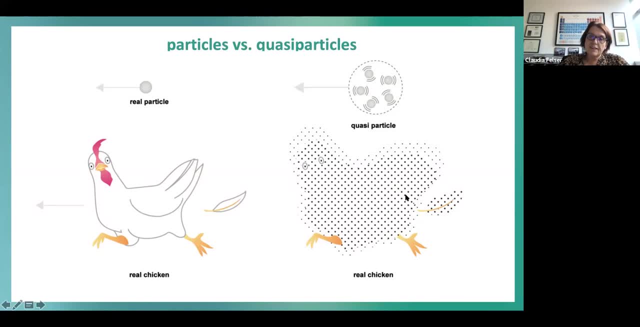 what we do in finance matter physics, and indeed they are. they are very interested in this because this could show them that the fundamental equations are making sense If you see it in model systems. So, and it might be an explanation then to maybe solve one of the big question, the asymmetry. 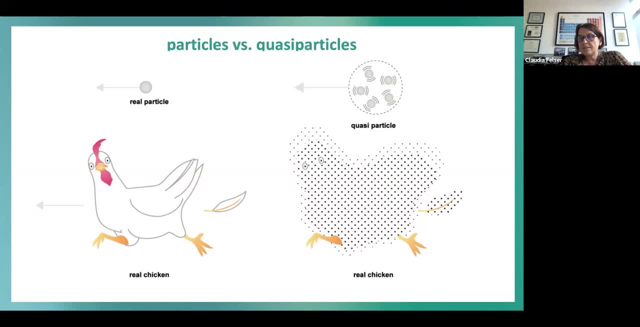 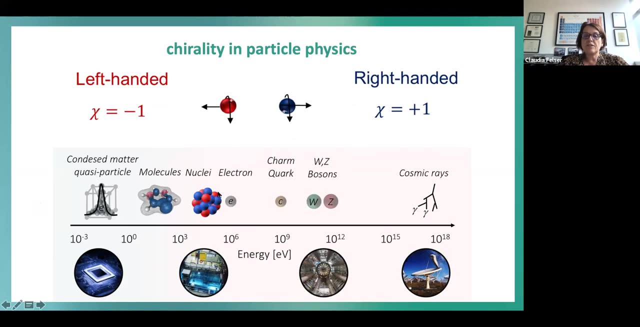 between particles and anti particle switches, more or less also the origin of our universe. Okay, so I have not the time, but this is also nice figure of of Johannes, very obvious, have to say. we have this symmetry baking in, in, in, in in the read: discussing and topological. 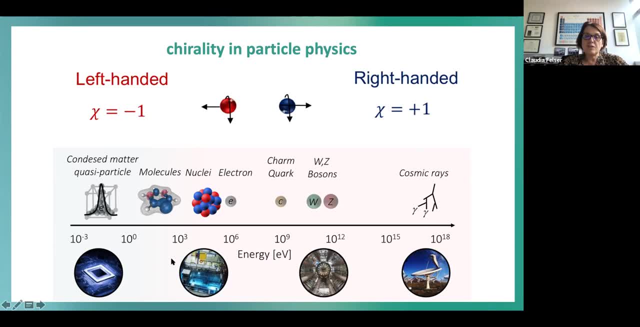 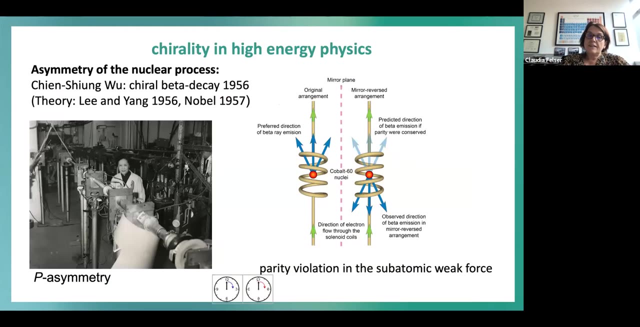 materials, but if you talk about astrophysics and if you talk about high energy physics, we are dealing with totally different energies, kids and also length skates, but still, I think it's very interesting to compare this different concepts. This is a So, so one similarity is like what is a, which is a similar parity violation, is the child. 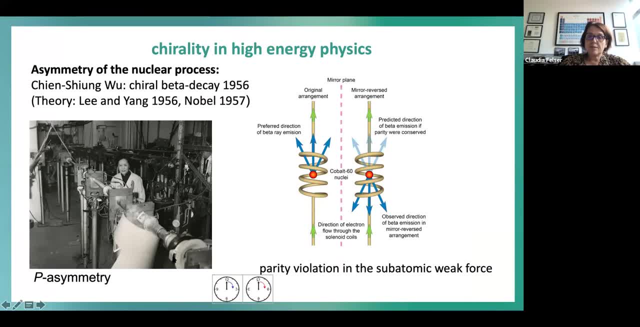 animal. So this is a similarity evaluation found by who experimentally in the better decay of of cobalt atom. so this is a It's related to the weak force and the nuclear, which is one way of explaining this asymmetry. and she should, she could show it in the better decay of cobalt and there was a theory. unfortunately, 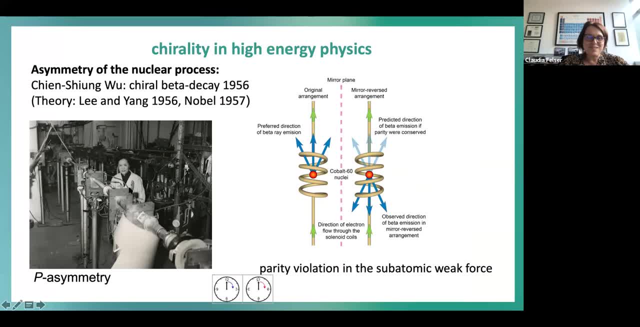 she didn't get the number price, only the theoretician. So good for you, Anyway, but it's very interesting here also. I show this example because it makes the bridge also this, this, this process: the weak force in, in in the weak force in in the nucleus. 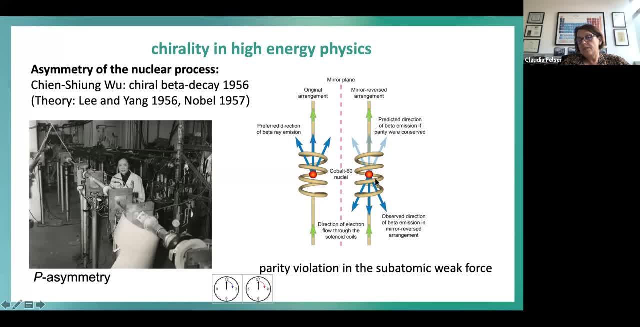 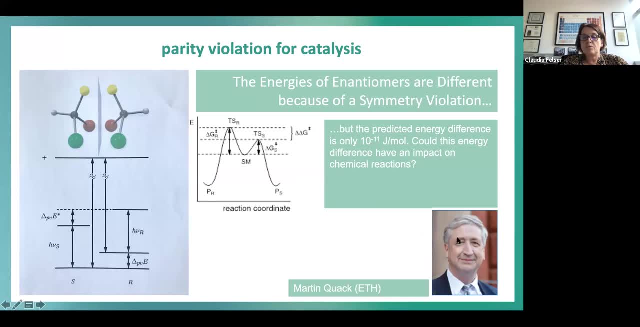 is nowadays even one possibility maybe to explain the asymmetry between the two charities. So this is connected with this guy. he's a professor at ETH search and he tries really to show That you can have, it can make a difference. so if you, if you take the weak force into, 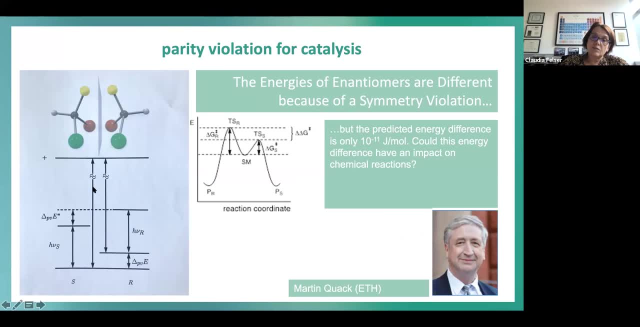 town. you should see it in spectroscopy. it could lead to a tiny asymmetry, that we get a tiny little bit more from one molecules and the SS, and this could be one possibility, for it could be one possibility to explain even the origin of life. 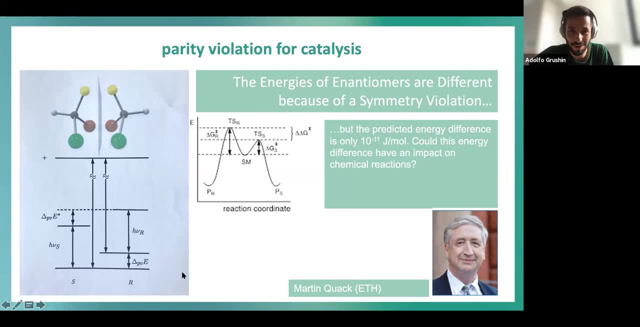 There's a question? Yeah, there's a question by Mikko. What other theorize the phenomena in high energy physics or maybe other areas could be realized? in condensed matter context, what would you like to see in particular? Yeah, so I have already some. 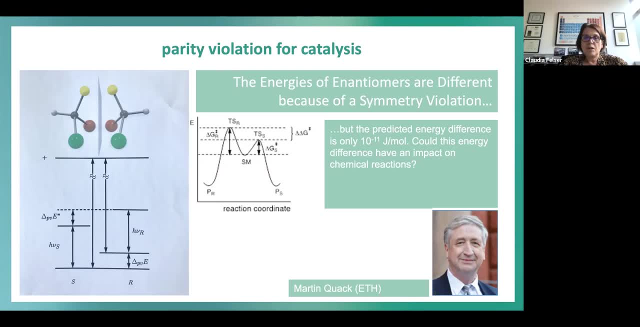 So you could ask this question also to our door for saying thank you, make it because I don't want. has given already a proposal and recently I got another proposal from Jen, So which is more related to optics. So, which is more related to optics. 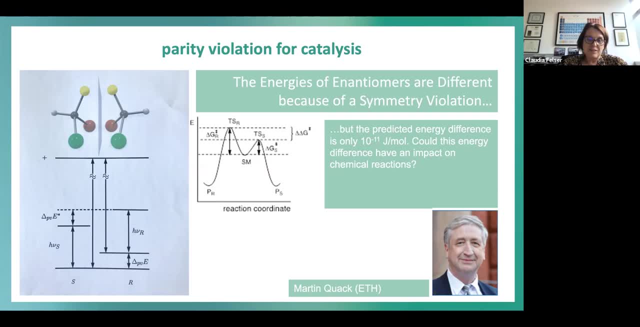 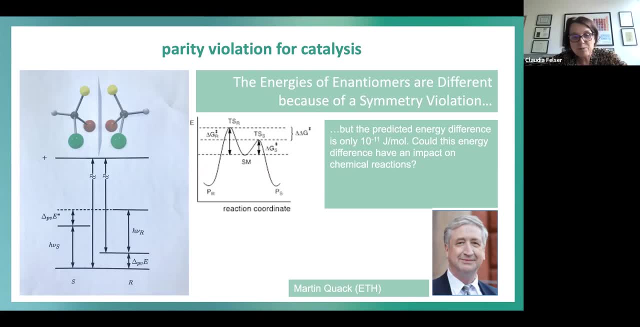 So, so, so, so, and we still dream about the horizon experiment and maybe you should talk also. we are going in a very good direction, so we are doing similar things. so we we find now more and better ways and different materials. so we have this child materials. okay, so which? 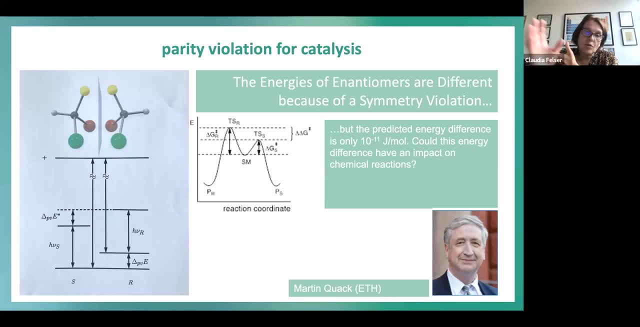 might open new direction And also the quantum Hall effect, The quantum fractional Hall effect and things like this might have. Anyway, so this is a very good question, but the question should be addressed to the theoretician. we already have a list of some things. okay, there's still the idea to show this negative. 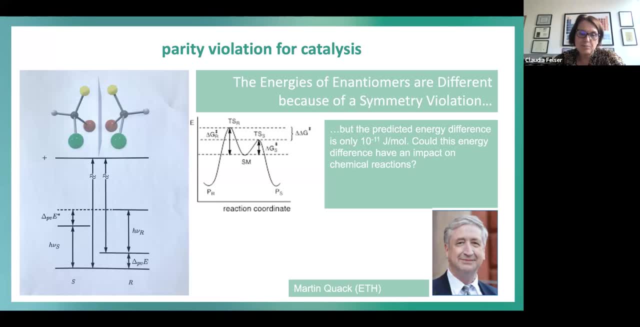 curvature horizon and the black hole experiment, and this is icing on the very urgent to do list of Johannes and us And yeah, so we are ready to wait for good ideas. Yeah, Okay, now is the twisted materials, and could even think: can we take twisted materials? 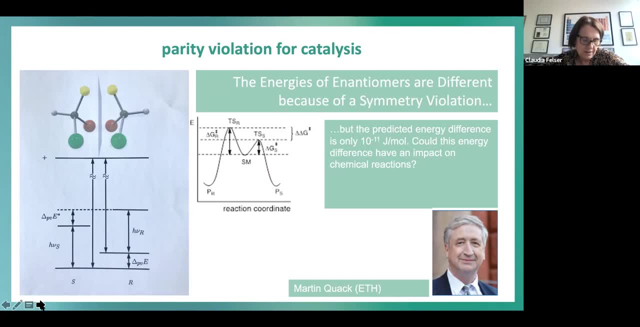 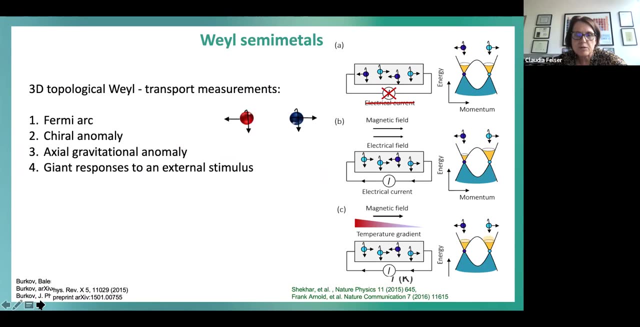 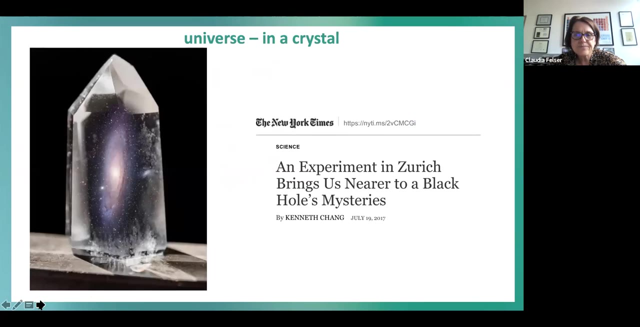 into account for doing some of this experiment. Okay, I think I'm running out of time and I think I will start with the vitamin methods and the experimental observation, maybe tomorrow. Then I want to go to the axion insulators and and I want to do a little bit of gyro. 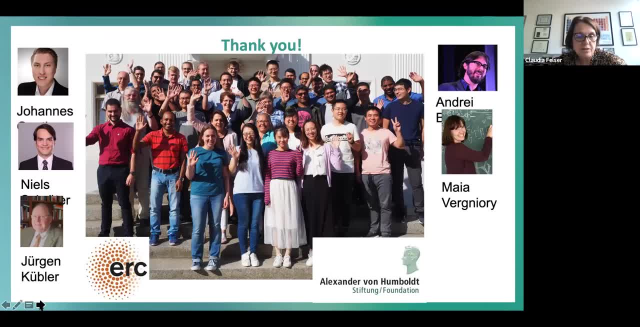 stuff And, if there's time, magnetism, but it might be not enough time, but I think I really give you a little bit of taste of the different direction to inspire the theory to do more, and there's another question. So very good. 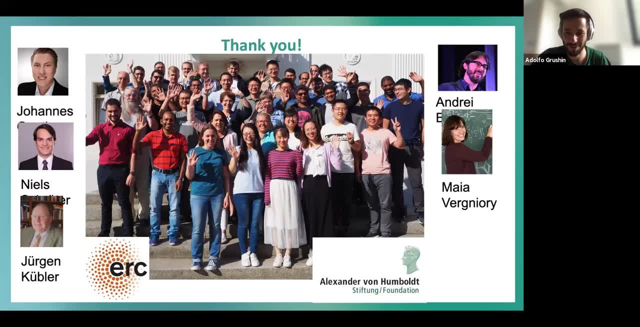 So thank you, Claudia, for your talk, Very inspiring. I'm going to take this other question. it's a clarification. I know, Okay, maybe this point was explained, that I missed it, but let me ask it: Can the presented chemistry based point of view give a nice interpretation of the obstruction? 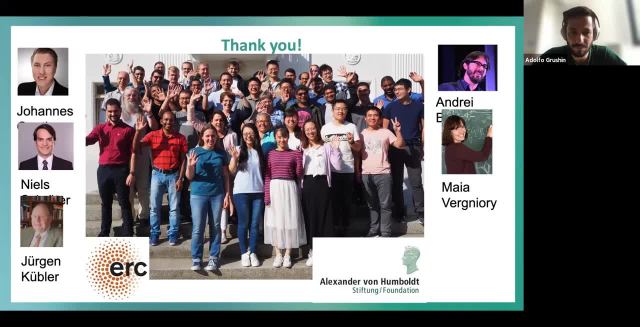 to having an atomic limit in the political insulators, The, the, the. I have to think about this. chemistry pays, chemistry based point of view to give a nice interpretation of the obstructed to having an atomic limit and top of the. I have to think about this. 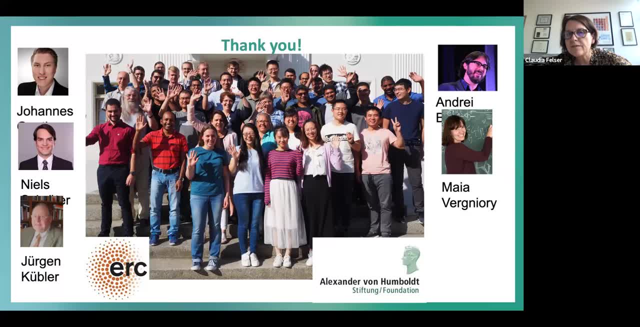 okay, I mean we need to discuss more with my about this. we were already. So I see this different group of obstructive atomic insulators, like the obstructive atomic insulators, and then the, the, the filling enforced obstructive insulators. I can explain. 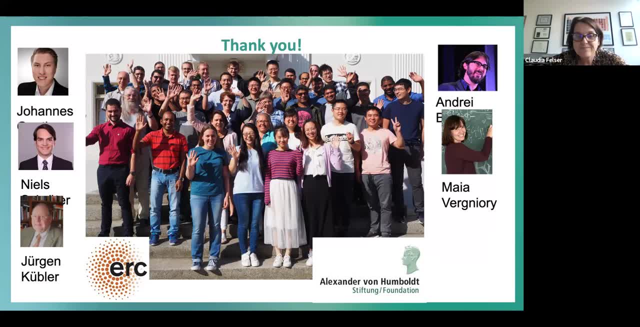 like the difference. I can explain by chemistry, But can I, can I explain the concept? I think there are some hand waving arguments in chemistry which simply takes experience into account, but this is a nice way to really bring it on some rational fundament. I would. 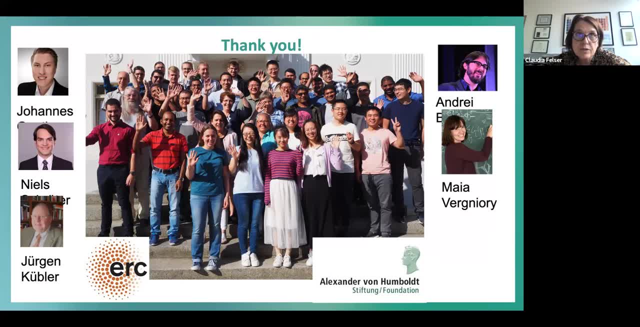 say So. therefore, I think from the fundamental viewpoint, it's not straightforward, But anyway. so it's a very good question. I could give another talk about this. I'm working on this for Maya and Okay, Very good. Any other questions I don't mind. I wanted to add something to this answer.